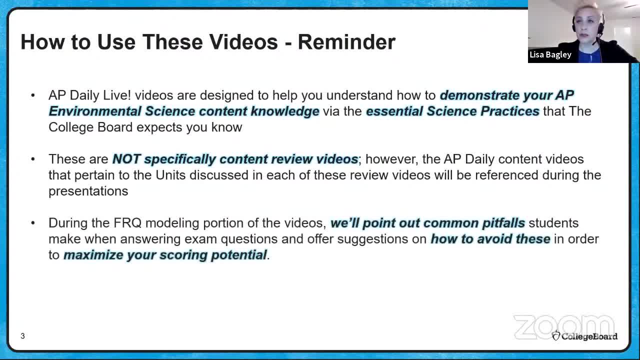 please feel free to reach out to me. I'll be happy to answer any questions you may have. During the free response modeling portion of the videos, I'll point out common pitfalls that students make when answering exam questions and offer suggestions on how to avoid these. 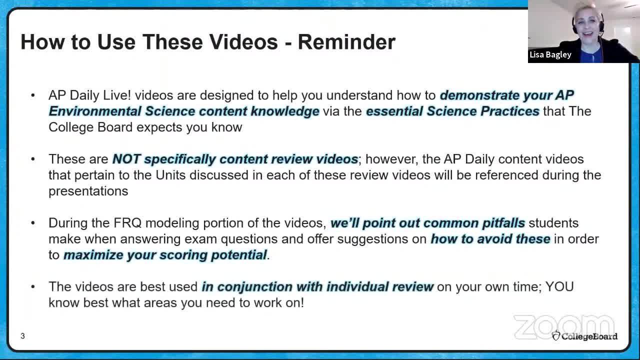 in order to maximize scoring potential. And, as always, these videos are best used in conjunction with your own personal review on your own time, because you know best what you need to work on. I shared these last night with you because I know you're going to love them. 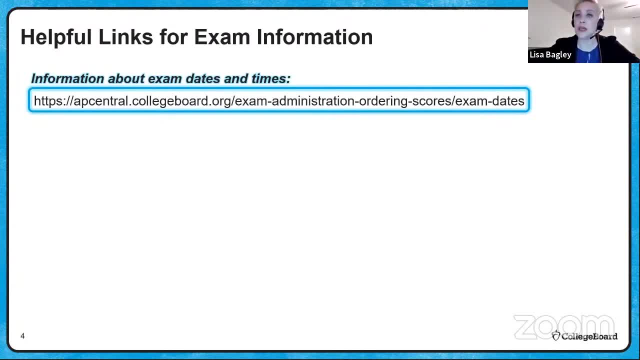 I'm going to share them again. These are helpful links for the AP exam information. So specific information about AP exam dates and times can be found at the following URL, And you may want to take some screenshots of these as we go through. Information specifically about our exam, AP Environmental Science, can be found at the: 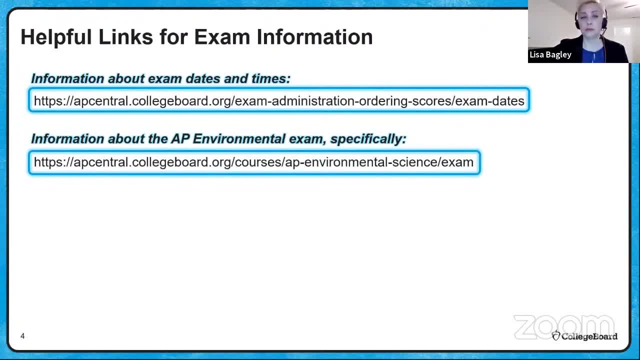 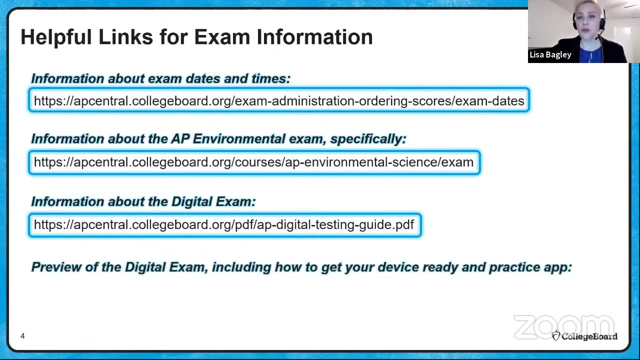 following URL: Information about the digital exam can be found on the digital testing guide, which is at this PDF. We're going to talk a little bit more about digital testing tonight, And a preview of the digital exam, including how to get your own device ready and the practice app, is available at this website. So again, if you need to take 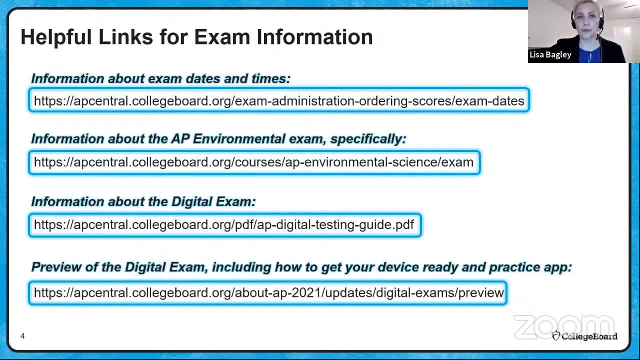 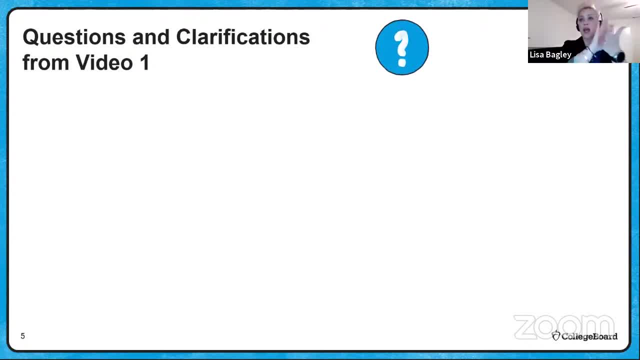 a screenshot. that's probably a good idea. So let's first jump into questions and clarifications from video one. First off, thank you so much for joining us today. If you have any questions or comments, feel free to ask them in the Q&A box at the bottom of the screen. 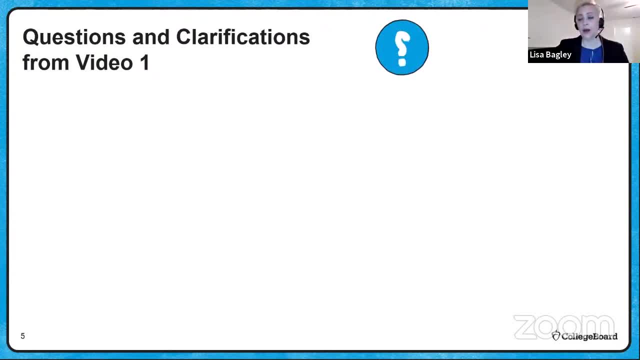 We've got a few questions in the Q&A box, So we're going to start with one. First off, thank you, my eco warriors, about giving me some feedback. Really, really, really want to say thanks for that, because the feedback is very valuable And it can make the videos better. So we're going to be 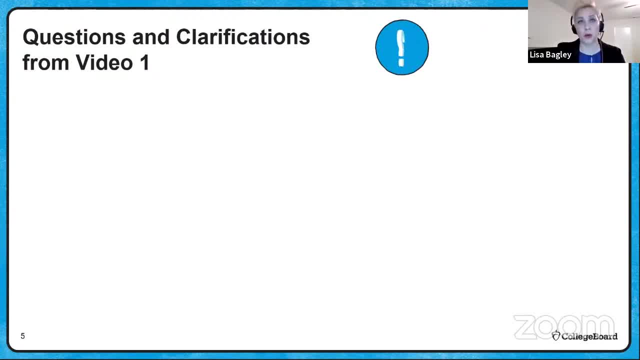 those are going to be actionable And I appreciate every little bit of feedback we got. So thanks so much for doing that. A lot of you all said hey, hey, we want more content review. I can understand that, But I want you to understand that the content is out there. friends, There's a lot of content in. 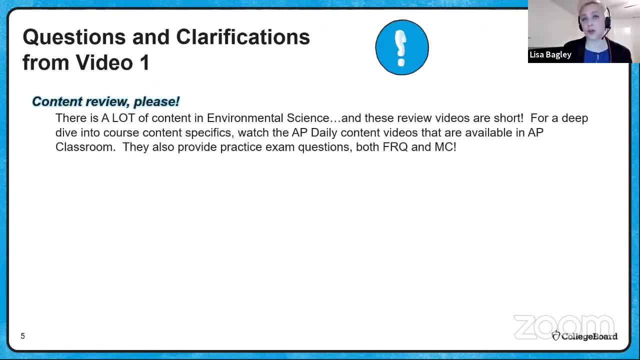 AP Environmental Science and Technology. So we're going to take a look at some of the things that you've seen in AP Environmental Science, And these review videos are short. If you want a deep dive into course content specifics, I'm encouraging you to watch the AP Daily content videos that are available. 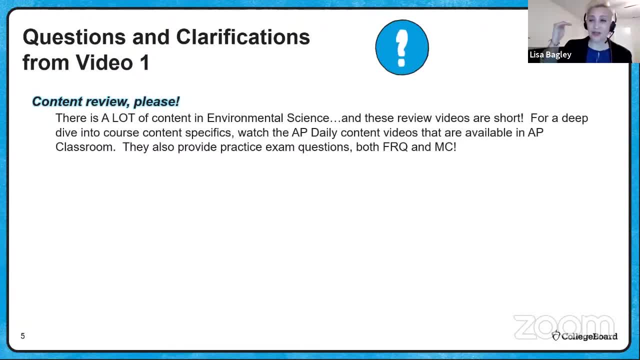 in AP Classroom. If you go into your AP Classroom account, they are there for you And they are deep dives into this content that we're talking about. They also provide practice exam questions for you, both free response and multiple choice. Check them out, please. I had questions on how long the 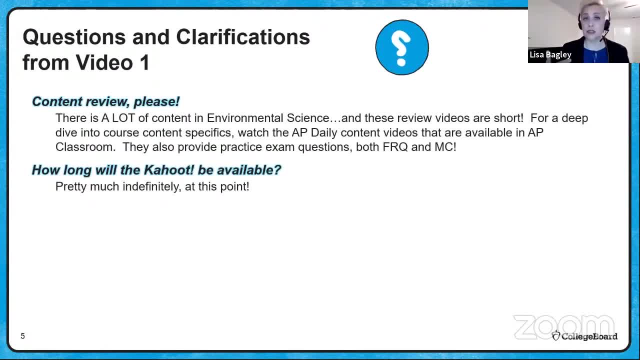 Kahoot will be available. Kahoots that are presented in these videos are going to be available pretty much indefinitely. right now, as far as I know, I don't have any plans to take them down, And so practice away. Lots of questions, also about real-time chat. Some of you guys 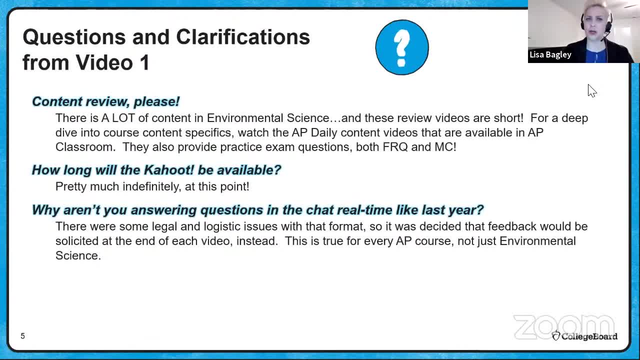 remember last year's exams. So there's questions: why aren't you answering questions in the chat real-time like last year? So there were some legal and logistic issues with answering the chat In real-time. so it was decided that the feedback would be solicited at the end of each video or 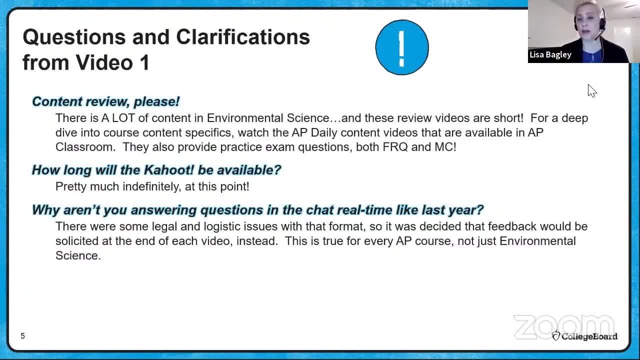 during each video, And that's what we did last night. We'll continue to do that. This is true for every AP course and not just environmental science. So if you're tuning into some of our other video series, you will also notice that the feedback is going to be solicited by Google Form. 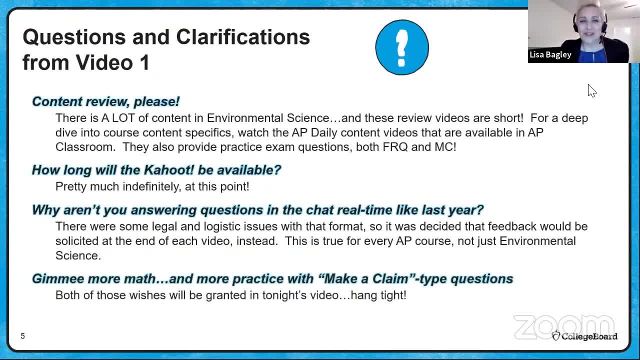 rather than live chat. Several of you wanted more math and more practice with make-a-claim type questions. Wish granted, We're going to be practicing some math and we'll be practicing some more make-a-claim type, which is science, practice seven. So hang tight, Let's keep going. Several of you wanted to know. 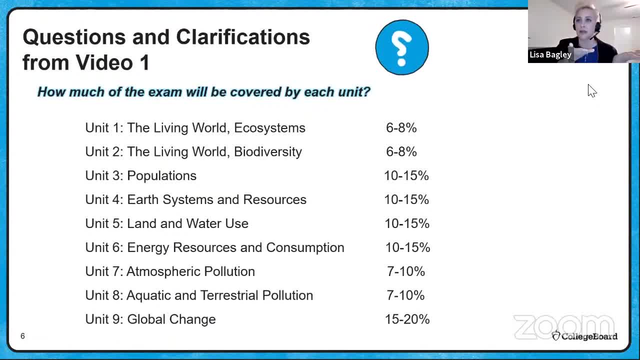 how much of the exam is covered by each unit. Ask and you shall receive. There you go. So each there's your units, one through nine, and how much of the exam content comes from those individual units. Take a screenshot, if you need to, so that you know which part is which. 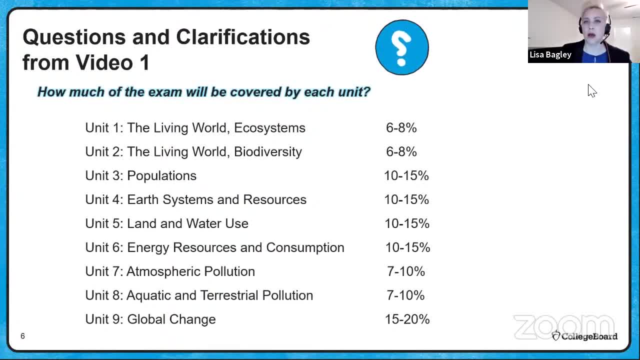 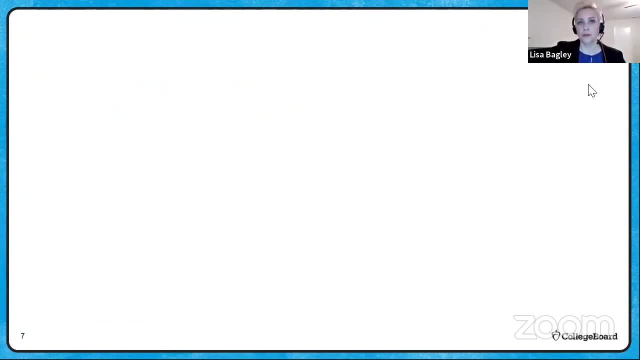 And you can see there that the first two units are six to eight percent. We move into about 10 to 15 percent for units three, four, five, six, seven to 10 for our pollution units and our biggie with global change at 15 to 20.. All right, So there were some questions about specifically. 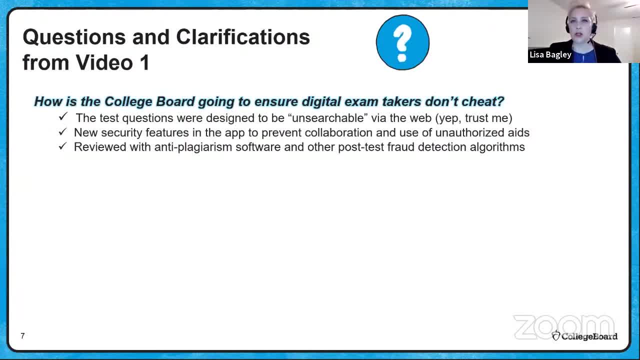 what's going on with the digital exam? How's the college board going to make sure that digital exam takers don't cheat? First off, not really my wheelhouse, but I'm going to tell you, this right, Some of the things we talked. 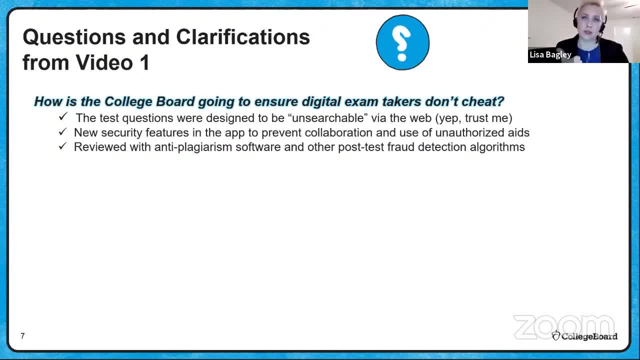 about last night. The test questions were designed to be unsearchable via the web, And when I say that, trust me on that one. We worked really hard to make sure that they were not searchable, So it's not going to be an internet search kind of thing. There's also some new security features. 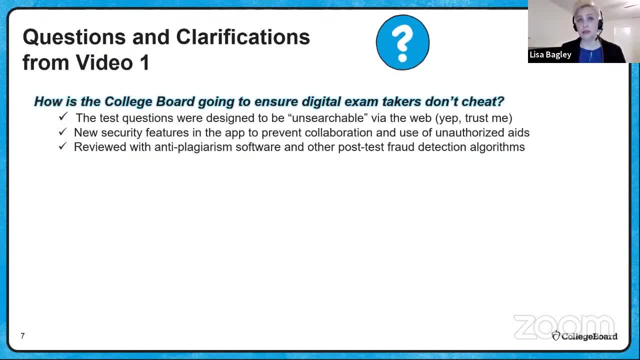 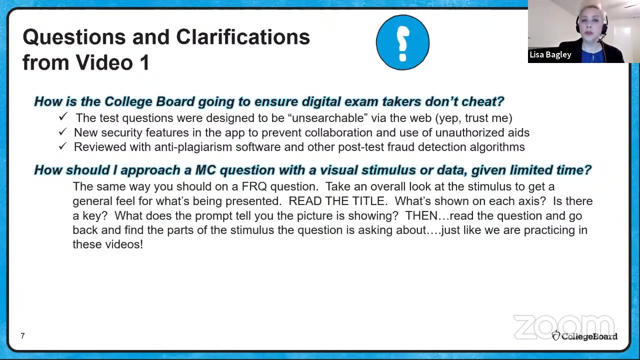 in the app to prevent collaboration and the use of unauthorized aids. And finally, the test will be reviewed post-exam with anti-plagiarism software and other post-test tests. So that's not going to be a big deal, All right. So here's the next one: How do I approach a multiple choice? 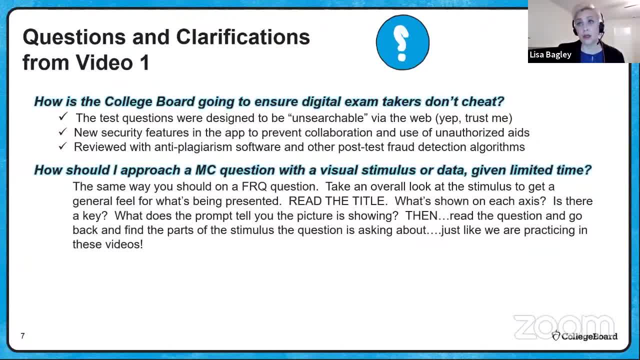 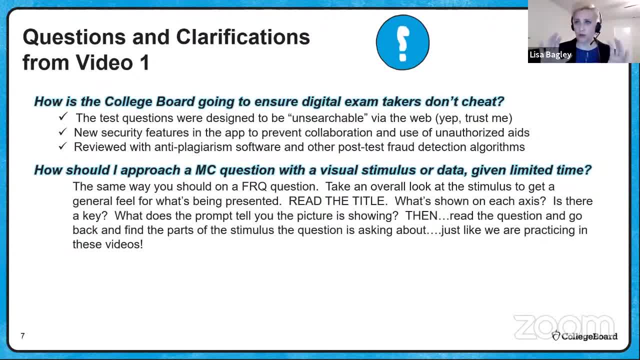 I always, when I talk to kids, I always say, hey, take an overall look at the stimulus that you're given to get a general feel of what's being presented. Read the title. What's shown, If it's a graph? what's shown on the axes? What's shown on the x-axis? What's shown on the y-axis? Is there? 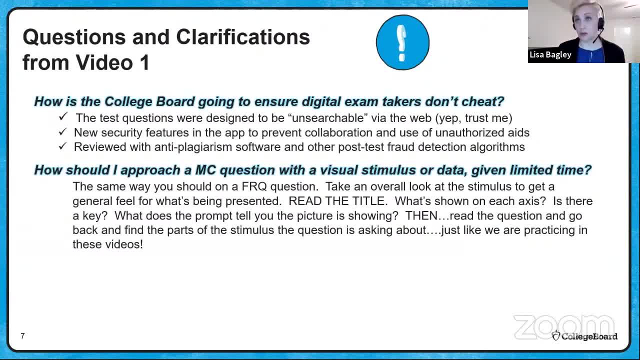 a key that goes along with it. What does the prompt tell you? that the image is showing or that the visual is showing? Then, once you kind of get an overall picture of what's going on there, read the question, Then go back and find the parts of the stimulus that the question is talking about. 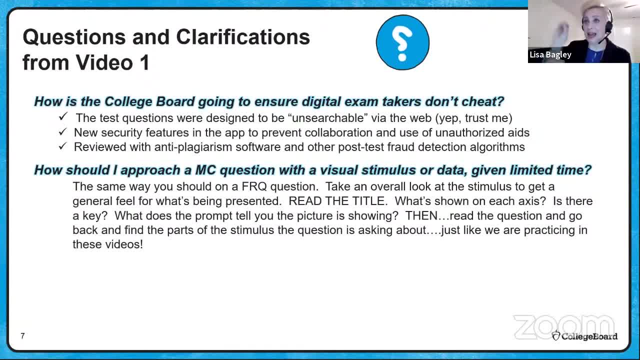 One of the things that we're modeling here is to read the stimulus and then go back and highlight: oh, they're talking about shrubs, or they're talking about demographic transition, stage two or whatever, just like we practiced in this video. So the strategies aren't any different. 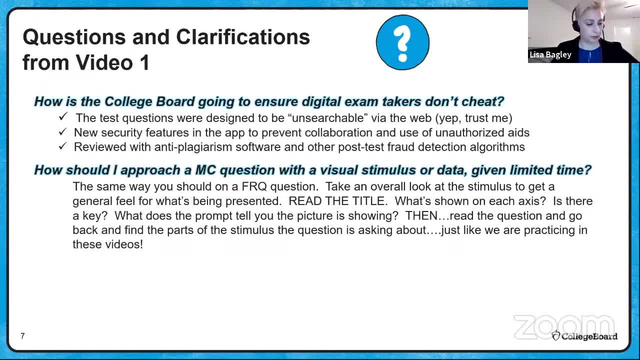 because, remember, you're timed on the free response portion as well. How much do I need to write for an identify prompt? Not much, friends, Just a complete thought that simply names or identifies the answer to the question. So it's an identify. 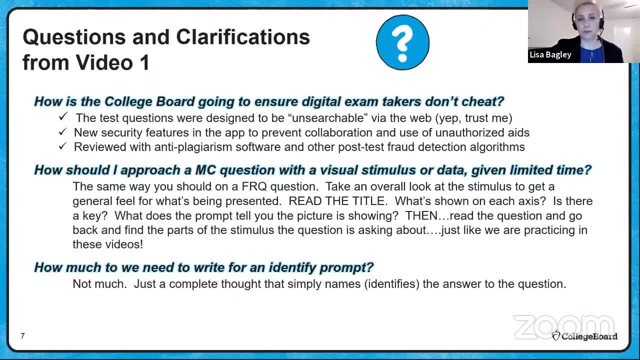 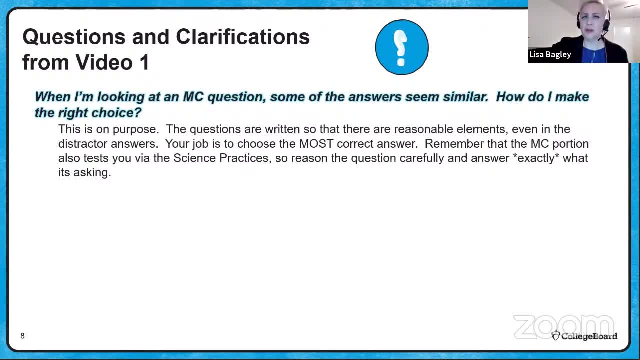 meaning just once you identify it. that's it. When I'm looking at multiple choice questions, some of the answers seem very similar. How do I make the right choice? Well, first off, thanks for saying this, because that's on purpose- The questions are written. 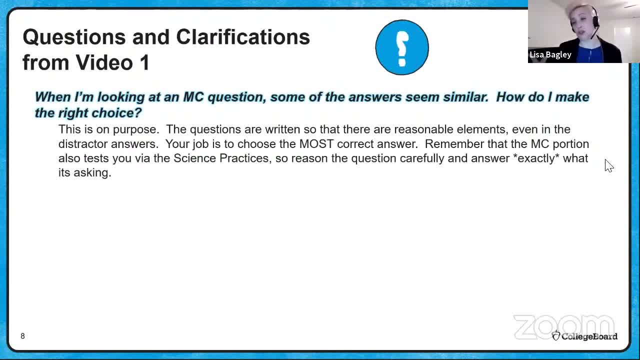 so that there are reasonable elements even in your distractor answers, meaning the incorrect answers. Your job is to choose the most correct answer. Remember that the multiple choice portion also tests you via the science practices, just like the FRQ portion. So read the question very. 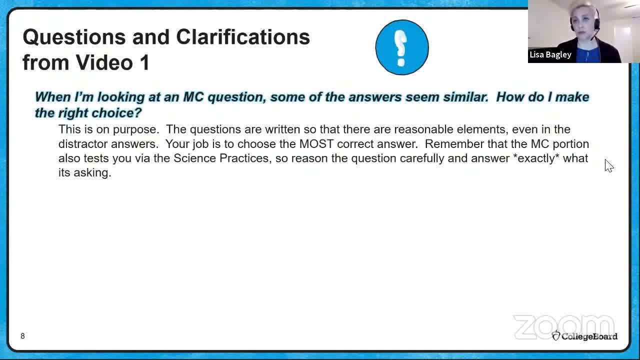 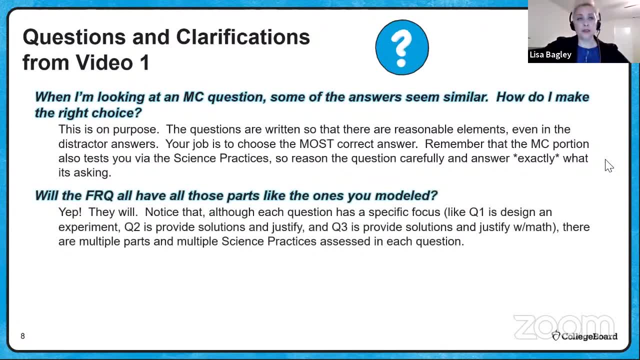 carefully and answer exactly what it's asking you to do. Those science practices flow throughout both sections of the exam. Will the free response have all of the parts, like the ones that you modeled last night? Yep, they sure will Notice also that although each question has a specific focus- like the question your question- one will. 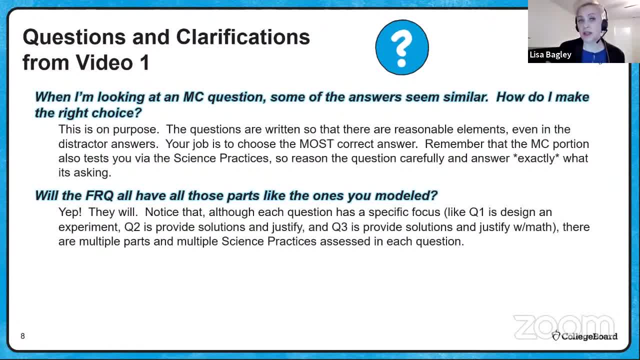 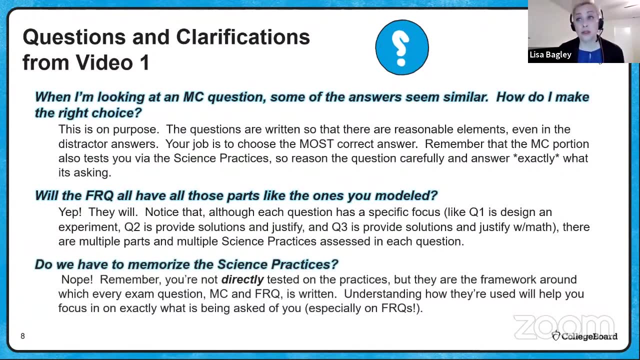 have elements of design and experiment. Question two will provide solutions and you'll have to justify those, And question three will provide solutions and you'll have to justify with math. There are multiple parts and multiple science practices assessed with each question. Do we have to memorize the science practices? 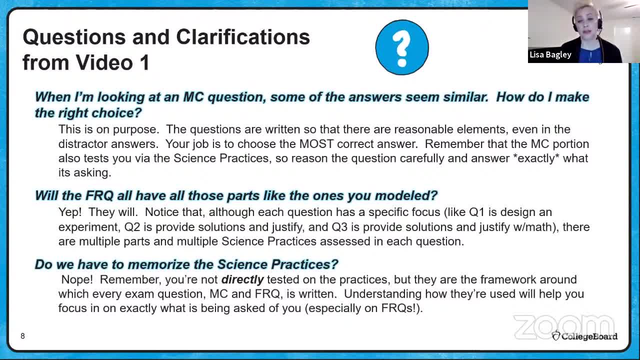 Nope, Remember, you're not directly tested on the practices, but I need to let you know that they are the framework around which every exam question, both multiple choice and free response, is written. Understanding how they're used will help you focus in on exactly what's being asked of you. 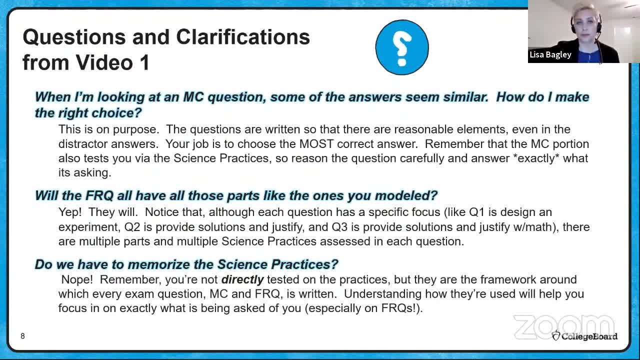 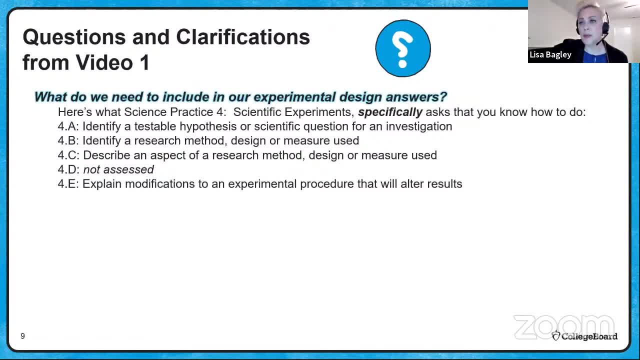 especially on free response questions: What do we need to include in our experimental design answers? Well, that's going to depend on what the prompt is asking you, but I wanted to share with you what science practice four, which is scientific experiments, specifically asks that you know how to do Science practice four A. 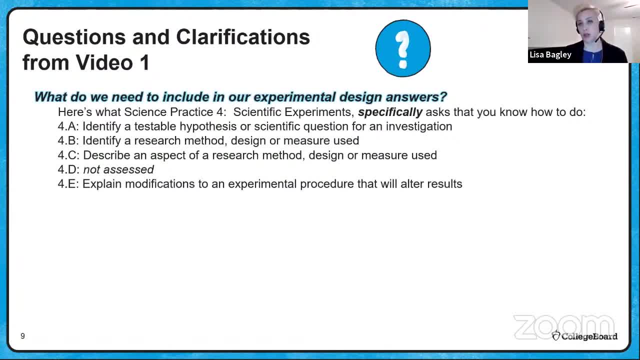 is: identify a testable hypothesis or research. question B is: identify a research method, design or measure used in an investigation. C is describe an aspect of a research method, design or measure used. So we've got two identifies and then a describe. 4D is not. 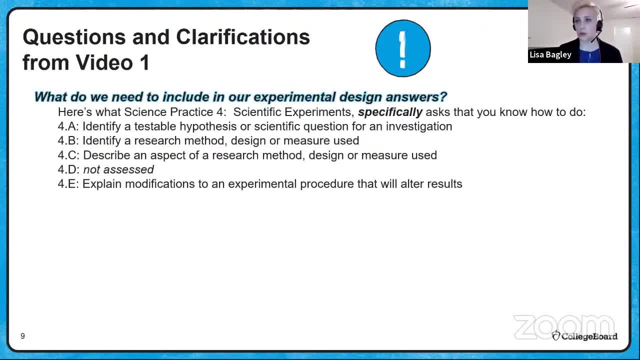 assessed on the exam. So we've got to identify a testable hypothesis or research. question 4D is not assessed on the exam. It's something that you would do in class. It has to do with experimental design in your classroom. And then 4E is explaining modifications to experimental procedures. 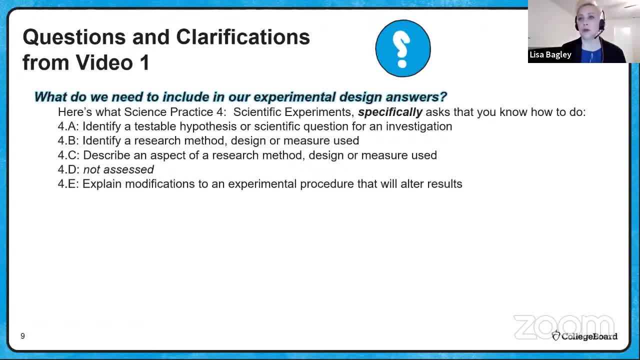 that may alter results. We had a little bit of practice with some of those last night. We'll have more as we go along through the video series. All right, Shout out to Brianna A from California. She asked about command verbs on the free response. 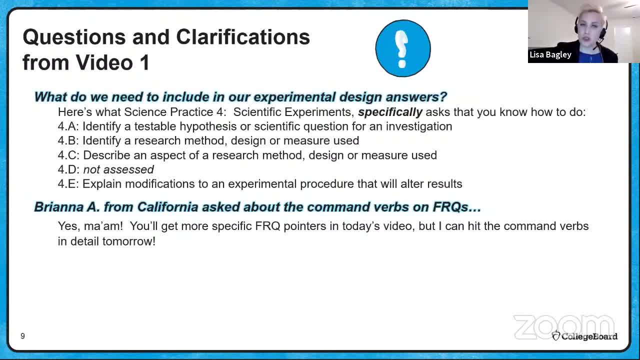 questions. Yes, ma'am, We will talk about those. You'll get some more specific free response questions in the next few minutes. So if you have any questions, feel free to reach out to me. I'll hit the command verbs harder in detail tomorrow, Like: how much do you need? What does? 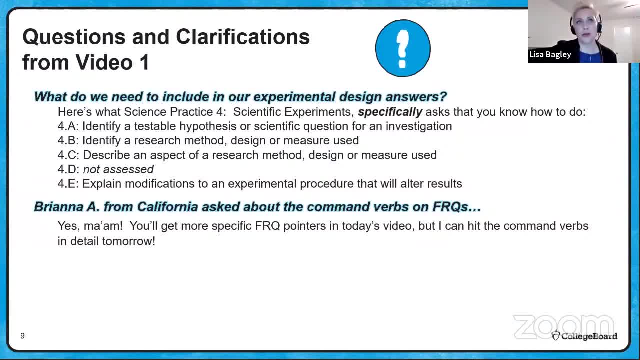 this actually mean for you to do All right. Tomorrow's video we'll have a little preview of all that wonderful stuff. Help, I'm freaking out about the biogeochemical cycles. Lots of you are freaking out about biogeochem. Don't freak out, my friends. Take a look at the AP Daily. 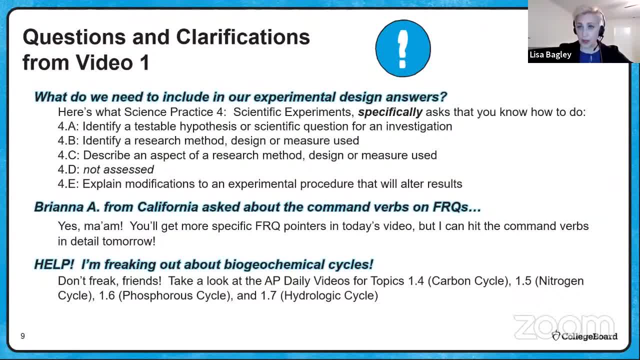 videos for topics 1.4,, which is the carbon cycle, 1.5,, which is the nitrogen cycle, 1.6,, which is phosphorus, And 1.7,, which is the hydrologic cycle. Those were done by yours truly and they are in depth. Now, what those don't cover is human. 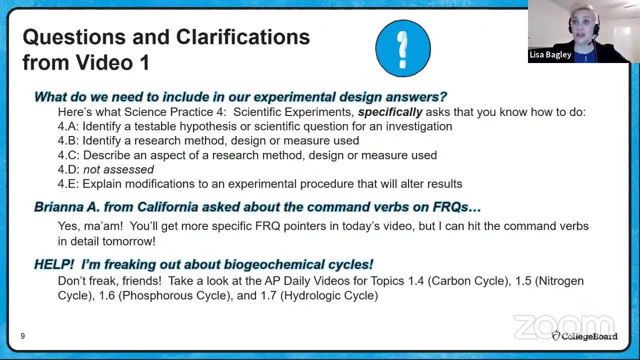 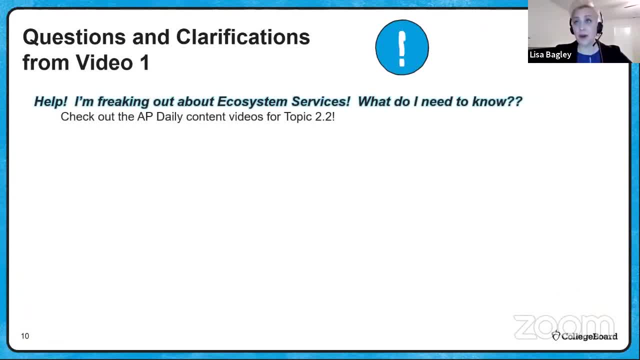 impacts, because that happens in later. But if you want to know the steps and the transformations, head there Help. I'm freaking out about ecosystem services. What do I need to know about those? There's a lot of questions about what's a different way to do it. I'm freaking out about 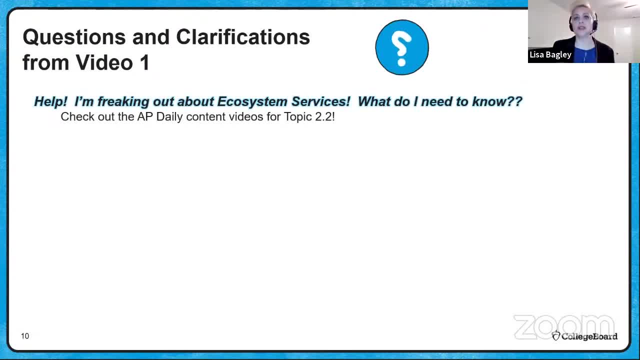 ecosystem services. What's the difference between a regulating service and a provisioning service? AP Daily content- video topic 2.2. Friends head there. There's a whole video series, three of them, on ecosystem services, And that's going to give you all you need to know. 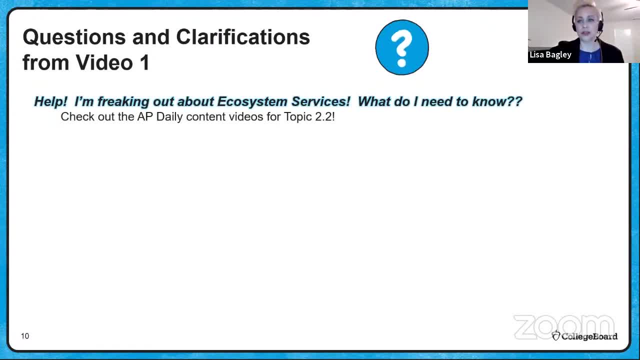 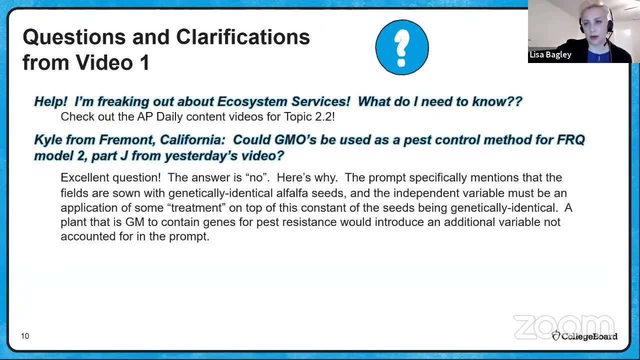 on ecosystem services and how they're used, both in the exam and content-wise. Kyle from Fremont, California, Kyle, you do not know how iconic Fremont is. He has a specific question about something I talked about yesterday. the second free response question: Could GMOs be used as a pest control method? 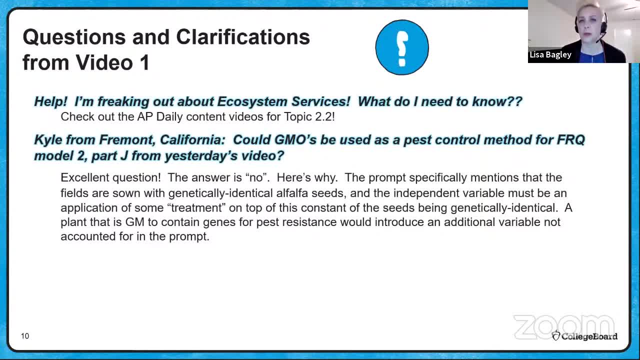 for free response: model 2, part J from yesterday's video: Excellent, excellent question, Very specific. I wanted to address that. The answer is no, Sorry. Here's why The prompt specifically mentions that the fields in the experiment are sown with genetically identical alfalfa seeds. 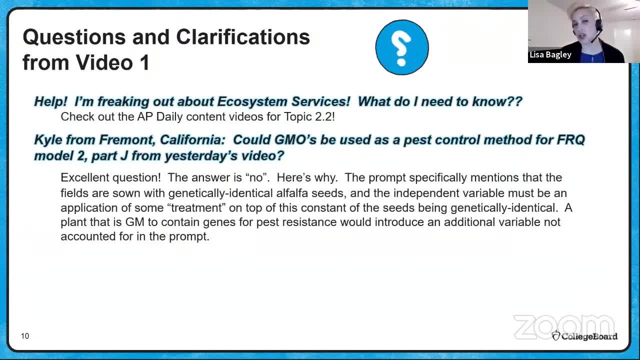 and the independent variable must be an application of some treatment on top of the constant that the seeds are genetically identical. So there's a constant there that the seeds are the same, They're genetically identical. A plant that is genetically modified to contain genes for pest resistance would introduce an additional variable, that is: 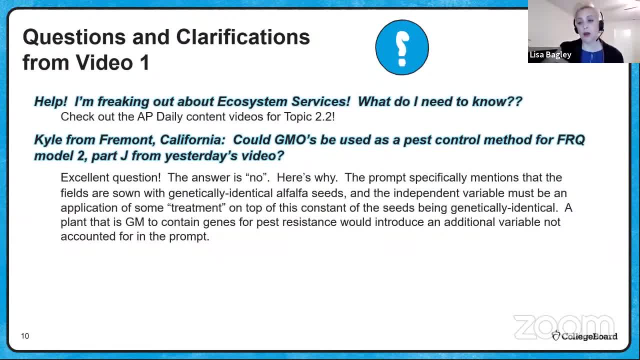 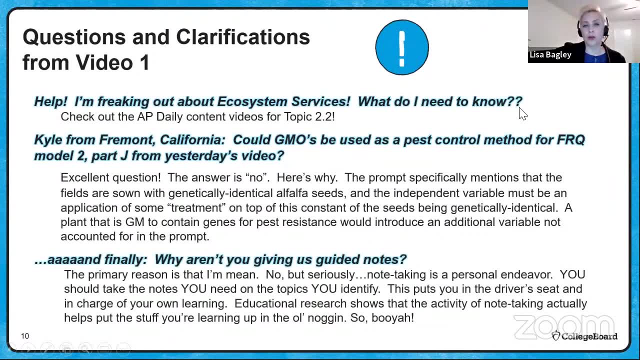 not accounted for in the prompt, So GMOs would not be a treatment for pesticide. I get where you're going and it's a great thought and I wanted to address it. And finally, why are you mean and don't give us guided notes? Well, the primary reason is, of course, because GMOs are. 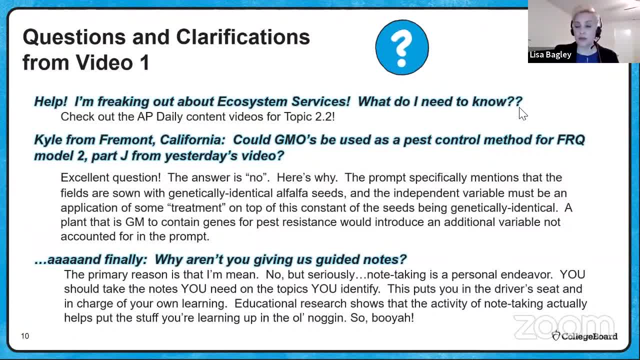 not a treatment. You can't use GMOs for a purpose. I think that's one of the most important reasons, of course, that I'm mean, But seriously, it's not. Notetaking my friends is a personal endeavor. 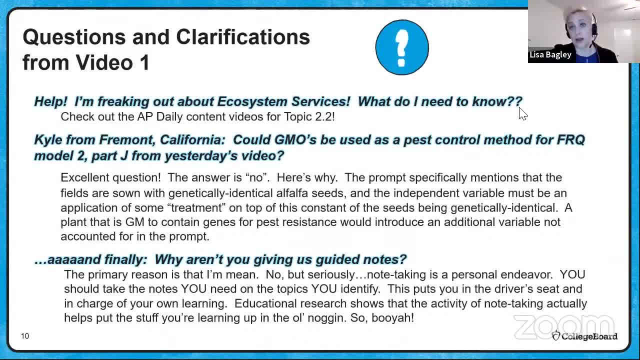 You should take the notes that you need on the topics that you identify as your weak points. This puts you in the driver's seat and in charge of your own learning. Also, I'm a teacher. Educational research shows that the activity of notetaking actually helps you put the stuff. 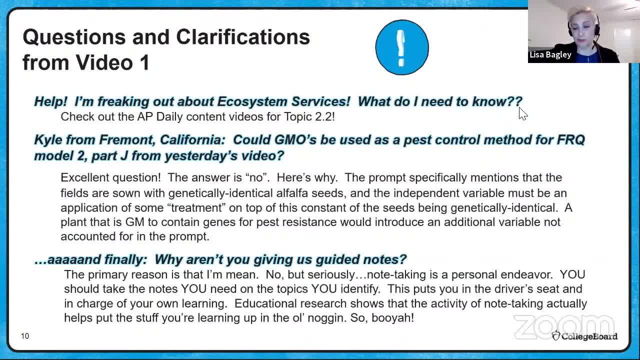 you're learning up here, So, booyah, take your notes. By the way, I'm just going to say something. At the end of this video series, there will be some guided notes given to you, but not before. Thanks, All right, so let's do some content review. 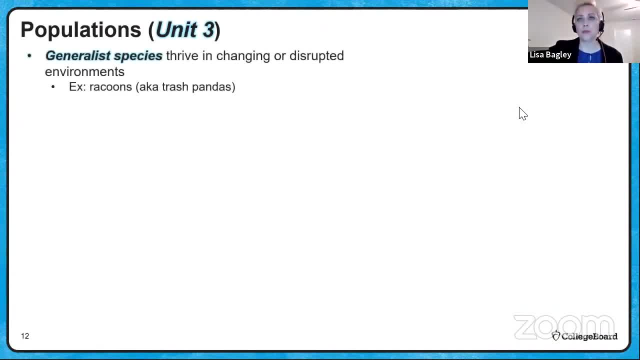 Jumping into populations, which is unit three: Generalist species. they thrive in changing or disrupted environments. An example of a generalist species would be a raccoon, sometimes called a trash panda. Specialist species are advantaged in environments that are stable, however. 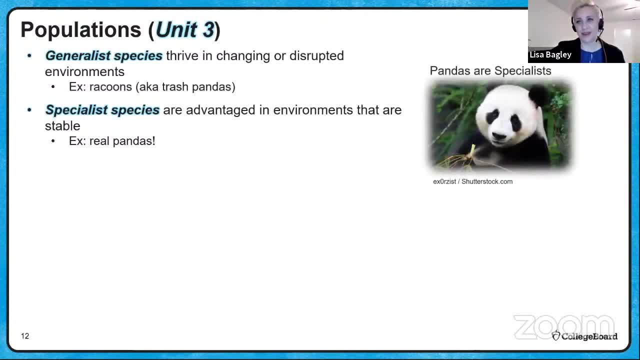 Example, there would be a real panda. Pandas are specialists. Our selected species are physically smaller. They have many offspring, They have early maturation and sexual maturity. They may reproduce only once during their lifetime, because their lifetimes are short and they have short. 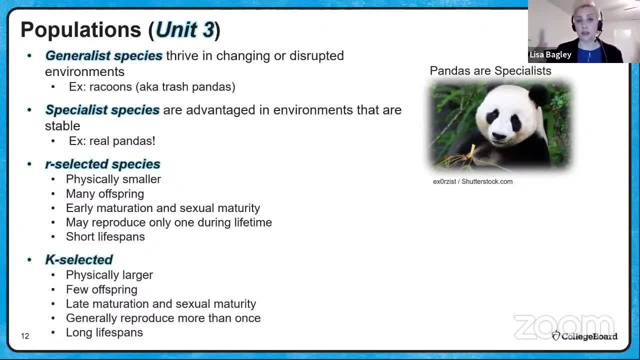 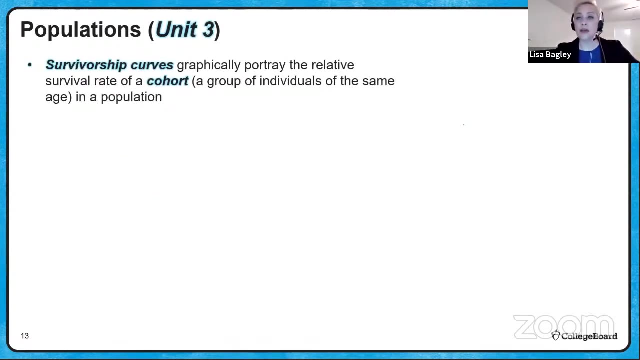 lifespans Okay. Selected species are physically larger. They have a few offspring. They have late maturation and late sexual maturity. They generally reproduce more than once during their lifespan. because they have longer lifespans. Elephants are case selected. Survivorship curves graphically portray. 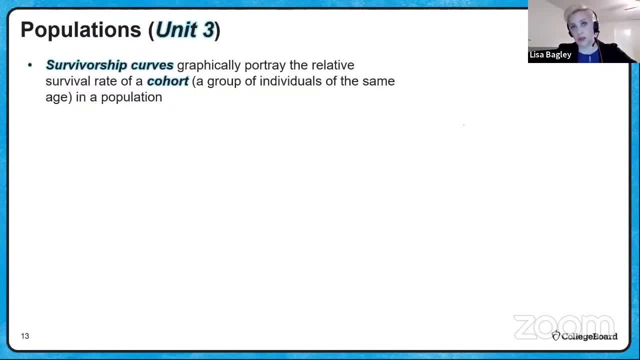 the relative rate of a cohort, which is a group of individuals of the same age in a population. They look like this: We have three types of survivorship curves: Type one, type two and type three. Type one curves show high early survival rates and increasing mortality with age. 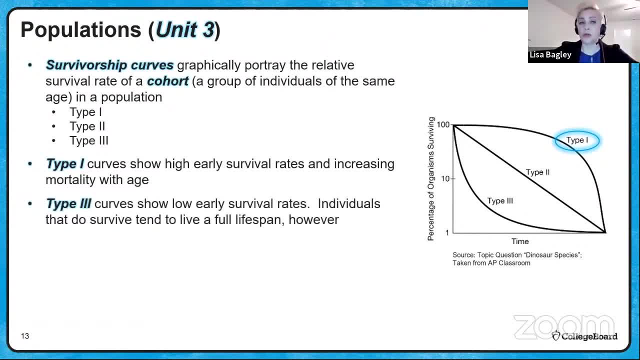 There they are right there. Type three curves show low early survival rates. Individuals, however, that do survive the early part of their lifespans tend to live a long life span. They tend to live a long life span. They tend to live a long life span. 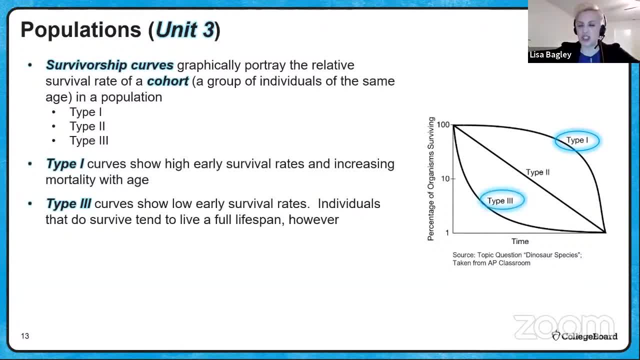 And there they are right. there It's kind of the inverse. Type one and type three are inverse. Type two curves show constant survival rates as the cohort ages And there's that linear line right there in the middle, R selected species generally follow type three curves. NK selected species. 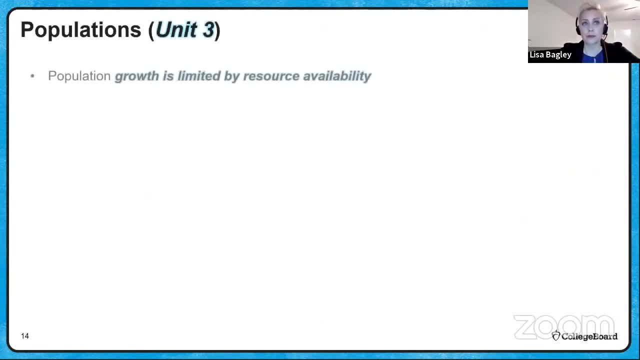 generally follow type one curves. Population growth will always be limited by resource availability, And resources are always finite. When resources are abundant, population growth increases When resources are scarce. unequal distribution in those resources may result in increased mortality events, decreased fecundity. What the heck is that? Oh, it's the ability to produce new offspring. 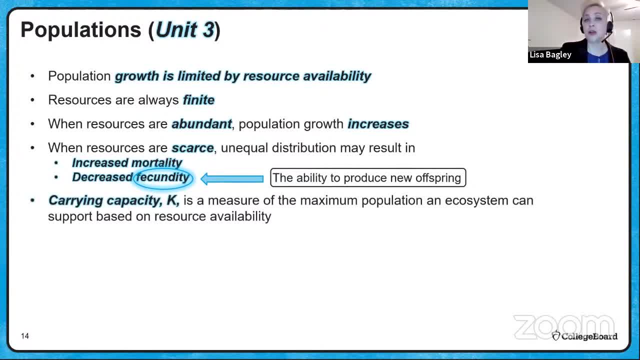 The carrying capacity, or K, is the measure of the maximum population and ecosystem can support based on resource availability. Overshoot refers to when a population exceeds the carrying capacity of its ecosystem. Overshoot can result in environmental consequences such as resource degradation or a dieback of the population. 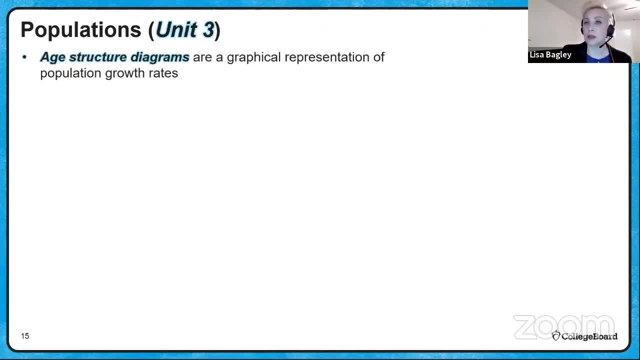 Age structure diagrams are a graphical representation of population growth rates. They look kind of like this, So we often see those in relation to human populations, but they can also be created for non-human populations as well. These diagrams have characteristic shapes depending on how quickly a population is growing. 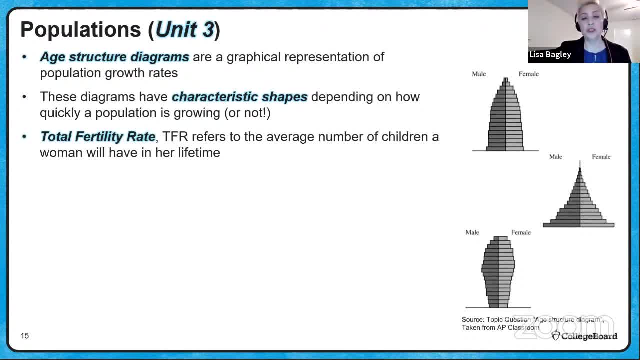 or not growing. Total fertility rate, or TFR, refers to the average number of children a woman will have in her lifetime. Total fertility rate is affected by the age at which a woman has a child, has her first child. educational opportunities for women. access to family planning. 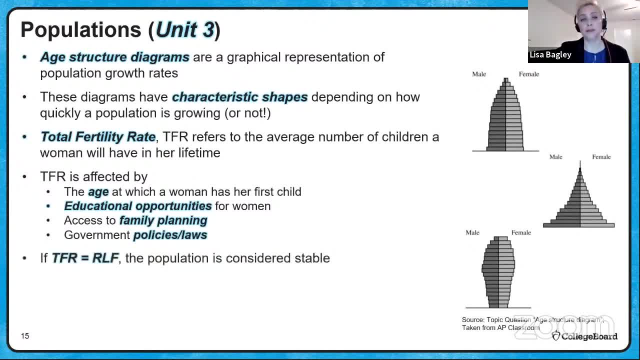 and government laws, policies and laws. If the total fertility rate is equal to the replacement level fertility, the population is considered stable. Normally that's around two. Infant mortality rate refers to the number of deaths prior to age one Child mortality would be deaths. 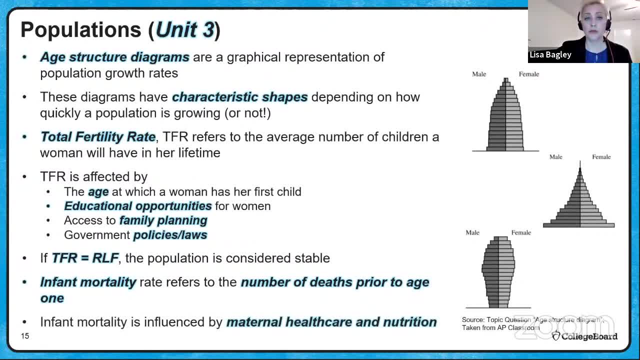 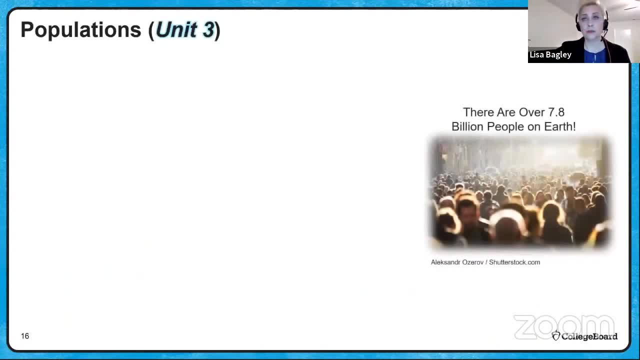 prior to age five. Infant mortality is influenced by maternal health care and nutrition. Guys, there's a lot of us on earth. There are over 7.8 billion people on the planet. Human population growth or human population decline in a geographic area is influenced by: 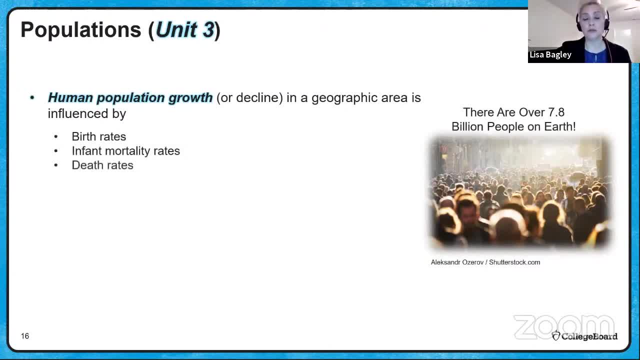 the birth rate in the area, infant mortality rates, death rates and access to family planning, as well as access to education and age at marriage. The earlier you get married, the more children you generally reproduce. On a global scale, human population growth. 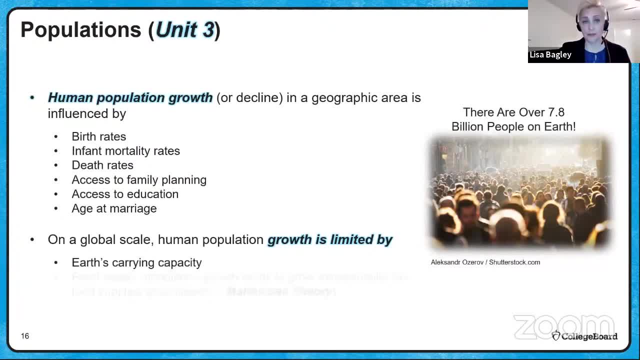 is limited by the earth's carrying capacity and food supply, So we're going to talk a little bit about this. Population growth tends to grow exponentially, but food supplies tend to grow linearly. This is called Malthusian theory After Thomas Malthus, and we'll talk a little bit more about that. in our practice, 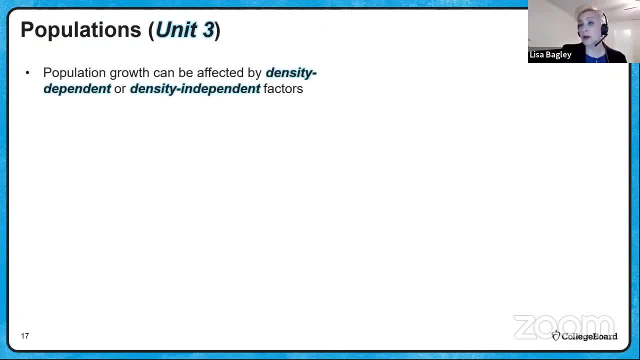 Population growth can be affected by density dependent or density independent factors. Density dependent factors include access to clean water, access to clean air, availability of food resources, disease transmission, territory size, density, Density dependent factors are types of factors that affect a population more as the population. 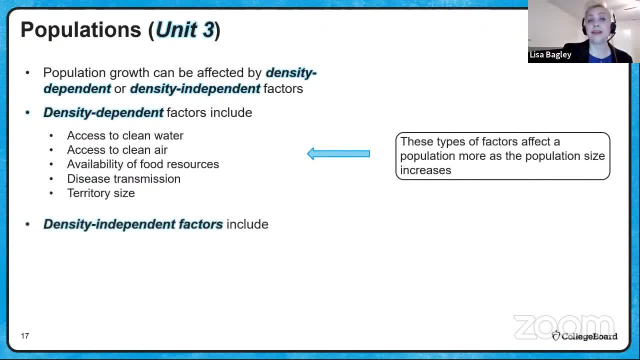 size increases Density. independent factors include major storms like hurricanes, tornadoes, tsunamis, et cetera, fires, prolonged heat waves and droughts. These are factors that affect a population at the same rate, no matter what the population size is, And you'll notice that there's 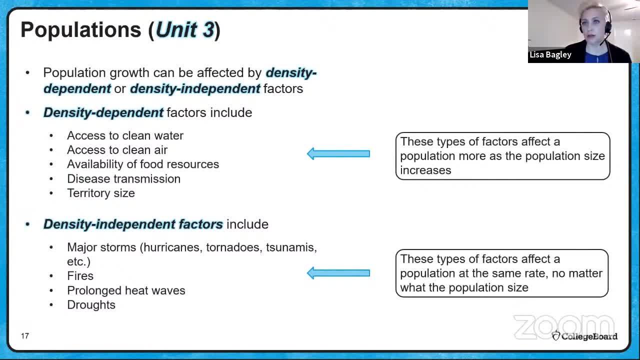 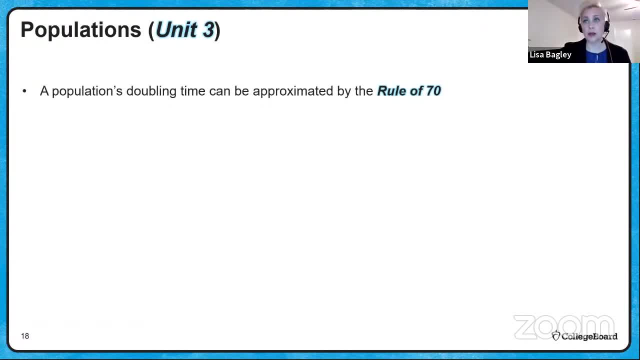 a little bit of a difference there. So these density independent factors tend to be abiotic. A population's doubling time can be approximated by the rule of 70.. Yay math, You're going to divide the number 70 by the population's growth percentage. The rule of 70 works for a population. 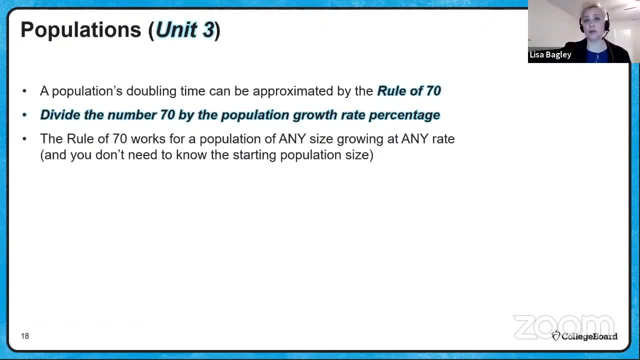 of any size, growing at any rate, and you don't need to know the starting population size. For instance, a population of approximately three hundred seventy-four thousand people is growing at a rate of 1.24% yearly. How long will it take for the population to double in size? 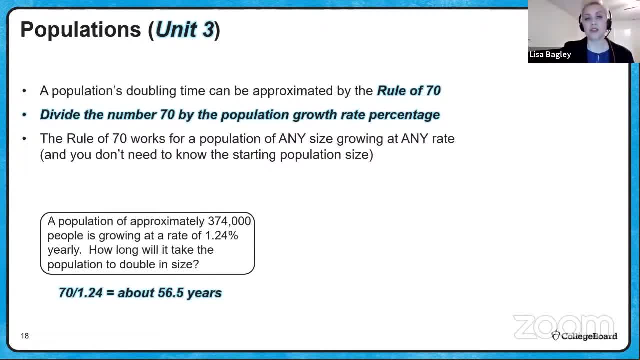 70 divided by 1.24 is going to double in size in about 56 and a half years. or if a population of reindeer doubles in size in 93 years, what is the growth rate of the population? 70 divided by x equals 93. So that's about a little less than 1% growth. 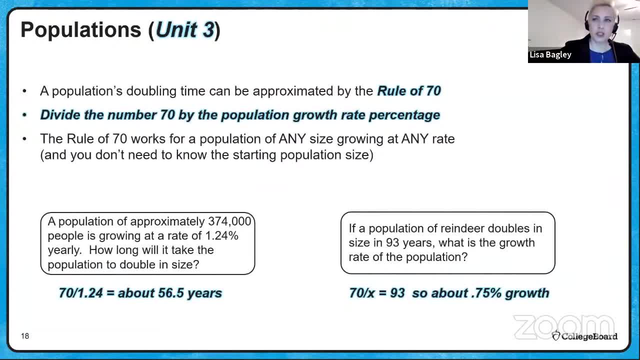 That's going to create a Transcendent Active Percentage Care Ecosystem. It's going to be a little less 75% growth. You always want to check this kind of math for reasonableness because if it's growing at 1%, then it should double in 70 years. So if it's growing higher than one, then your doubling. 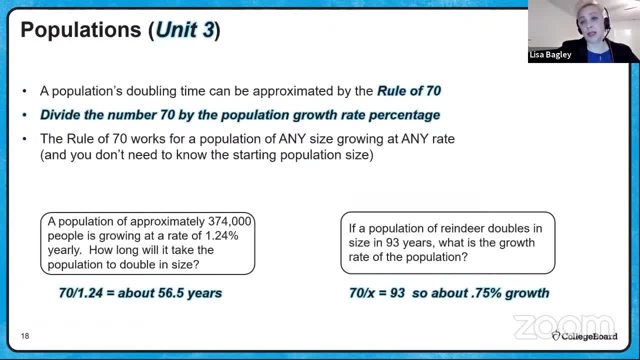 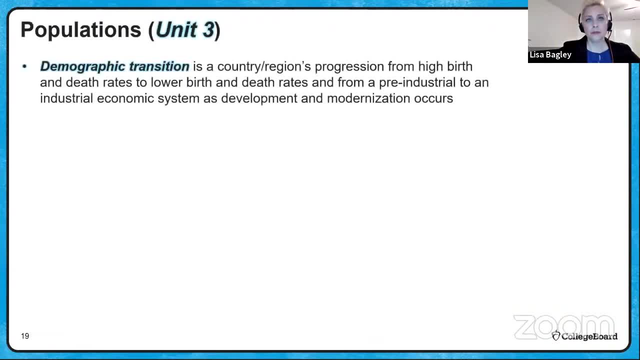 time will be less than 70.. It's growing. if it's doubling in more than 70, then your population, then your growth rate should be less than one. Demographic transition is a country or region's progression from high birth and death rates to lower birth and death rates and from a pre-industrial 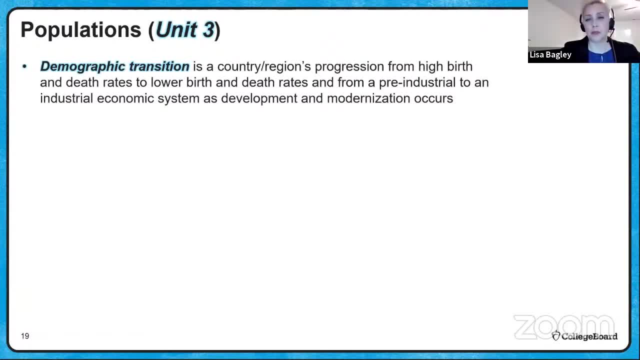 to an industrial economic system as development and modernization occurs. Characteristics of developing countries include higher infant mortality rates, more children in the workforce, lower life expectancy, lower rates of access to modern medicine and to education, and lower rates of access to safe drinking water and sanitation. 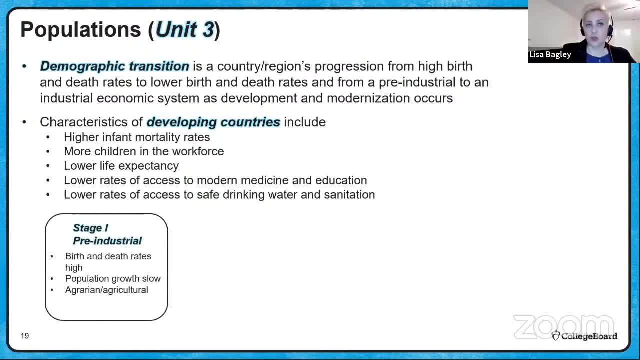 So we're going to go ahead and check this out. We're going to go just quickly through those stages. Stage one is your pre-industrial stage. Birth rates and death rates are high, Population growth is slow and the population tends to be agrarian or agricultural. 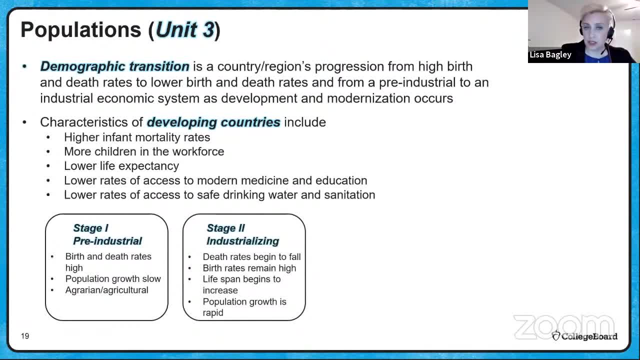 Stage two is our industrializing countries. Death rates begin to fall, but birth rates remain high. Lifespan begins to increase and population growth is rapid here. Stage three of demographic transition is your pre-industrial stage. Birth rates begin to fall. Death rate remains low from stage two, where it dropped. 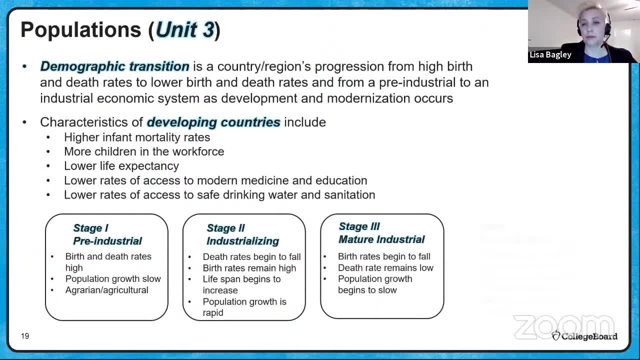 and the population growth begins to slow down. Finally, we have stage four, our post-industrial. Our birth and death rates are both low. The population is aging. When we're talking about age structure diagram, we have a higher proportion of aging or elderly individuals. 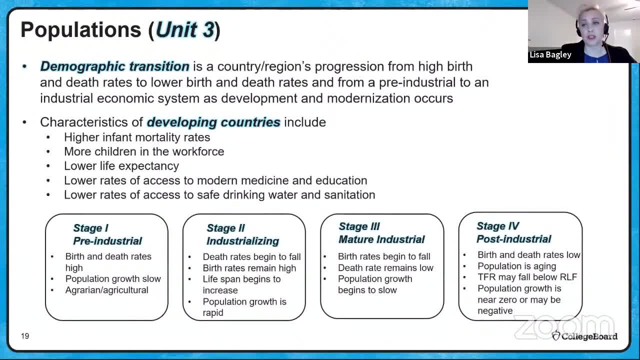 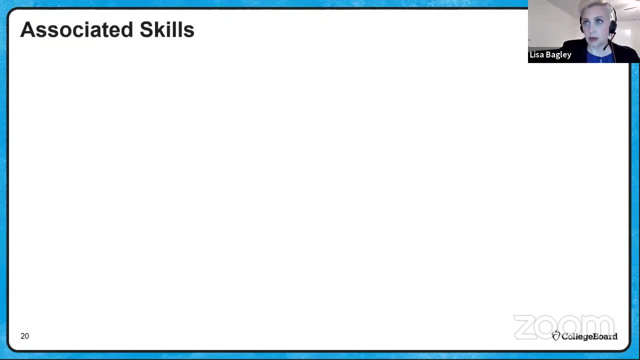 Total fertility rate may fall below replacement level. fertility and population growth is near zero, or it might actually be negative. We're going to practice with the visual model of those stages in a free response question. today Let's talk about the science skills that are associated with unit three. 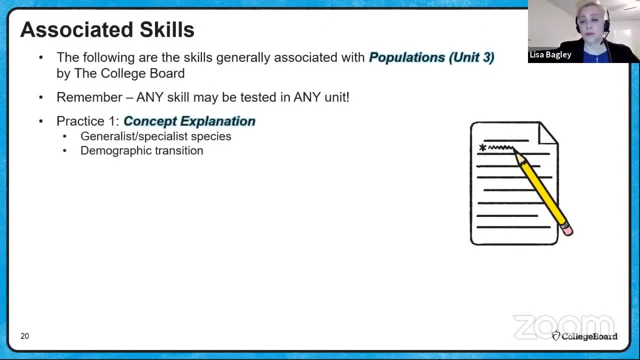 Remember, of course, that any skill can be tested in any unit. So for practice one, which is concept explanation. the College Board says that the generalist and specialist species and demographic transition can be associated with the concept of explanation. So for practice one. 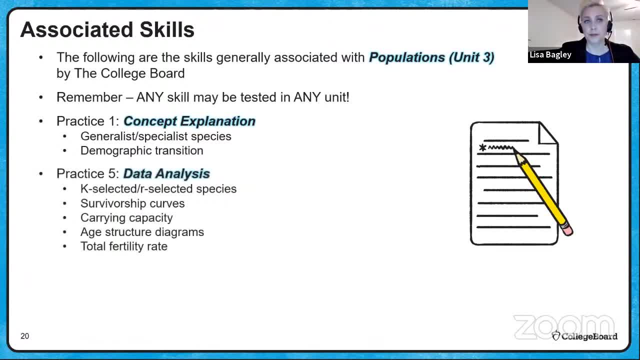 we're going to practice with the visual model of those stages in a free response question today. Practice five could be data analysis case selected in our selected species: survivorship curves, carrying capacity, age structure diagrams and total fertility rate. Practice six: mathematical routines: population growth and resource availability. 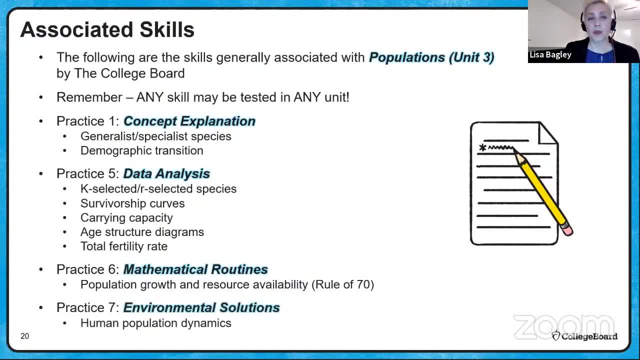 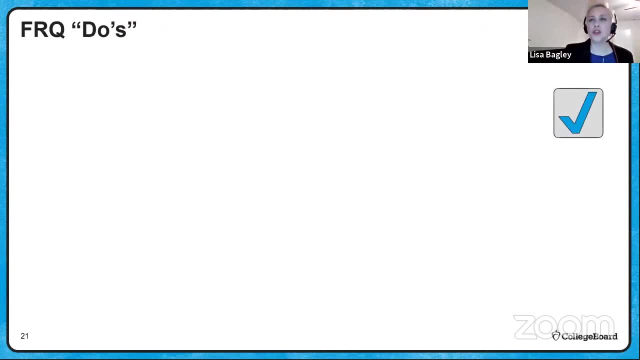 which is the rule of 70. And practice seven. environmental solutions, human population dynamics- We'll practice with several of these today. All right, let's talk a little bit about things to do when we write free response. questions that are going to be easier to point and things to do that make pointing an FRQ more difficult. 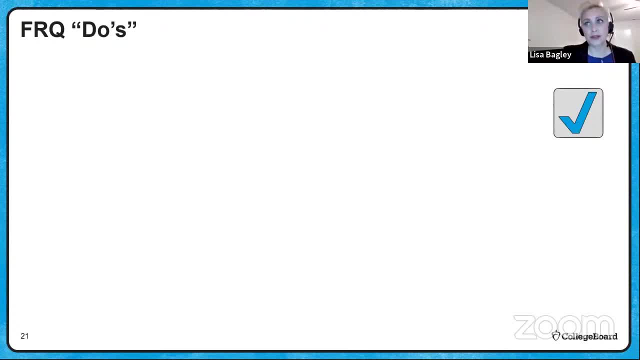 for a reader. This is going to help you get some of those points that you want on your free response questions. So as you read your prompt and take it apart for what the prompt is actually asking, you do dive right in to answering that question. You do have 23 minutes per question, so you need 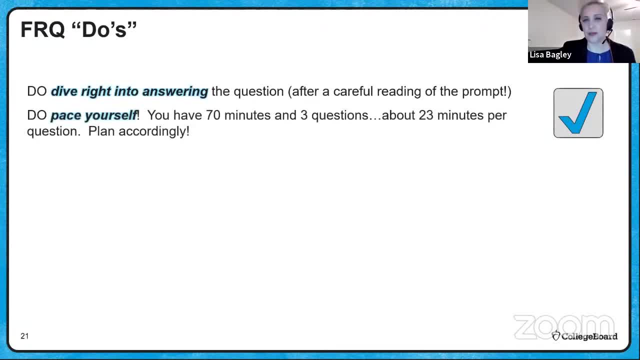 to use your time wisely, Pace yourself, of course. 70 minutes, three questions, about 23 minutes per question, so make sure you're planning accordingly. Remember, if you're a digital test taker, you can't go backwards and forwards, so you need to keep that in mind For paper exam takers. 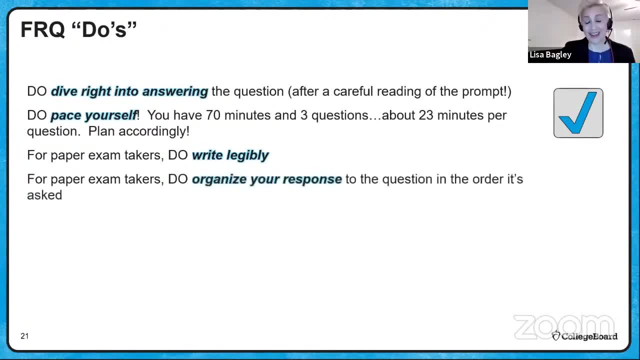 please make sure you write legibly And again for paper exam takers, please make sure you organize your responses to the question in the order that it's asked. Is this essential? No, Does it make it easier to read? It? does Do answer in complete thoughts. You don't necessarily have to have. 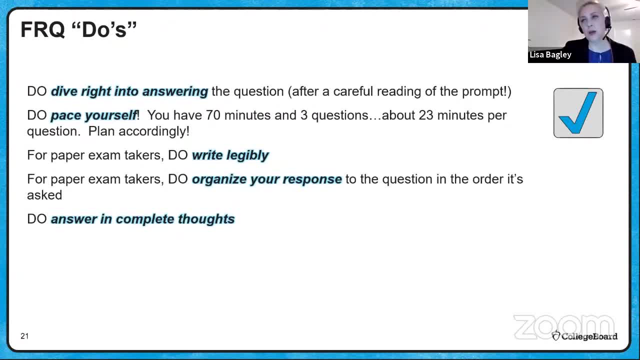 complete sentences, especially on those shorter prompts which are identify, but complete thoughts allow your reader to know kind of what you're thinking. Please elaborate with specific examples where they're asked. Please show your math units everywhere If there's a calculation. 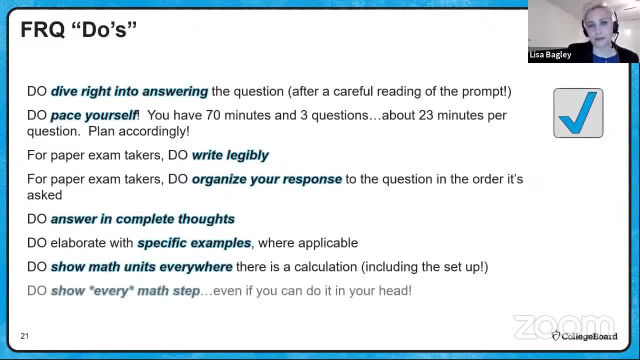 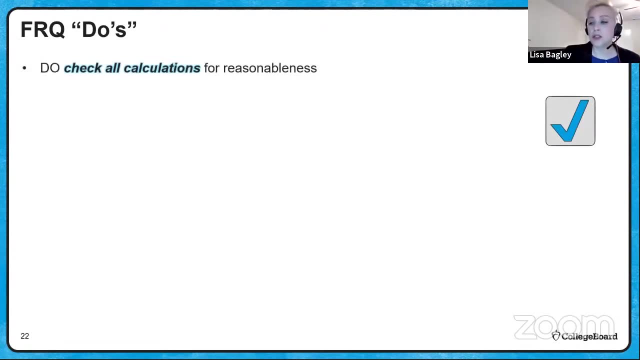 show your math everywhere, including in the setup, And show every math step. even if you can do it in your head- and a lot of you can, you're smart people- put it on the paper or put it into your digital testing app with units. Please check all your calculations for reasonableness. That's a. 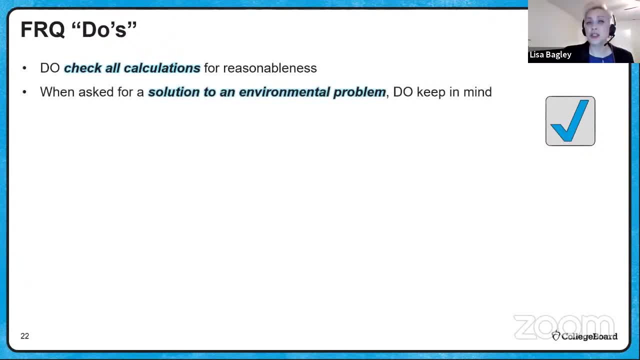 biggie. When you're asking for a question, please show your math units everywhere. If there's a calculation, they're asked for a solution to an environmental problem. Keep in mind the practicality and reasonableness of your solution And what type of solution the question is asking for, Is it? 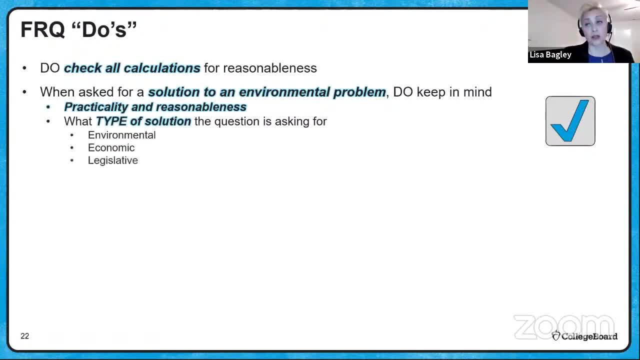 asking for an environmental solution, An economic solution, A legislative solution, A social solution. Make sure that you read carefully so that you're specifically addressing what they're asking. Do read and follow the instructions in the question carefully, If the prompt asks for. 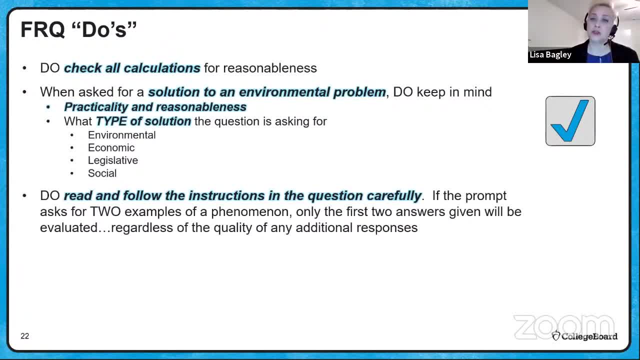 two examples of a phenomenon: only the first two answers that are given will be evaluated, regardless of the quality of your additional responses. So please make sure that you read: if they ask for two, give me two. If they ask for one, give one, because the additional ones 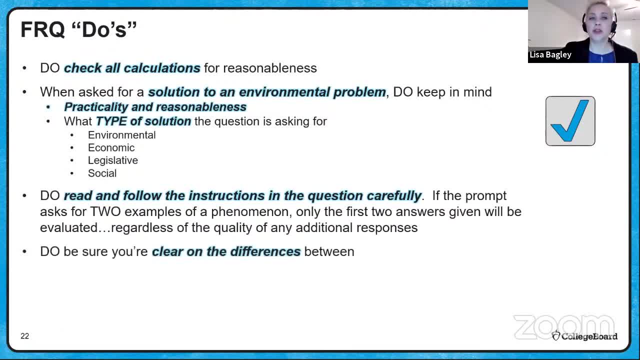 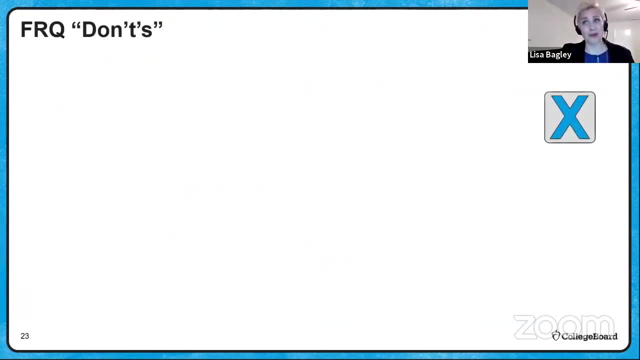 are not evaluated, And do make sure that you're clear on the differences between an environmental effect, an economic effect, a social effect or a human health effect. Okay, let's talk about some things that it would be better not to do. on a free response. 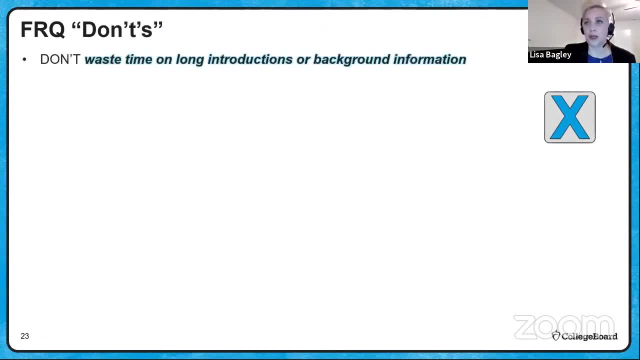 Please don't waste your time on long introductions or background information Unless the prompt specifically asks. please don't do that. Don't use absolutes like everything will die or everything will go extinct. Those are usually not true and they're usually not pointable. Don't use vague. 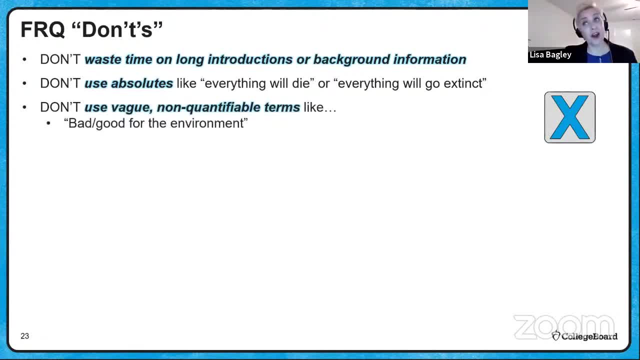 or non-quantifiable terms like that's good for the environment or that's bad for the environment, Or this hurts human health. If it hurts human health, be specific as to how. Or green, that's a green solution, Environmentally friendly or eco. These are non-quantifiable terms. They're usually 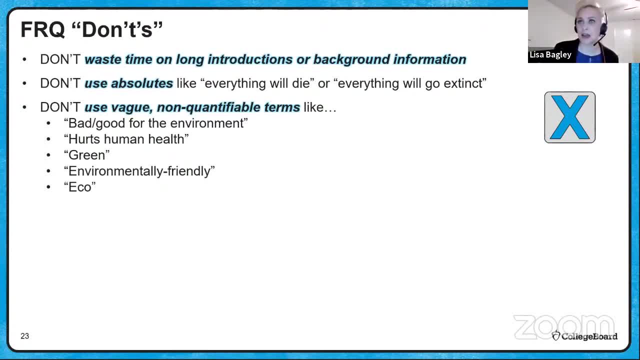 not specific enough to answer what the prompt is actually asking for. Don't write in first person. Don't use your name in your response. Don't use your teacher's name in your response. Don't use my name in your response And don't ramble. 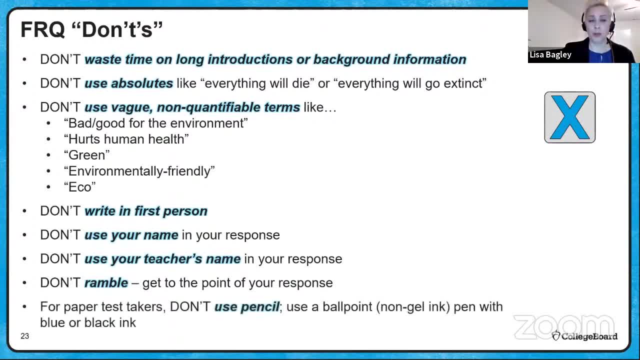 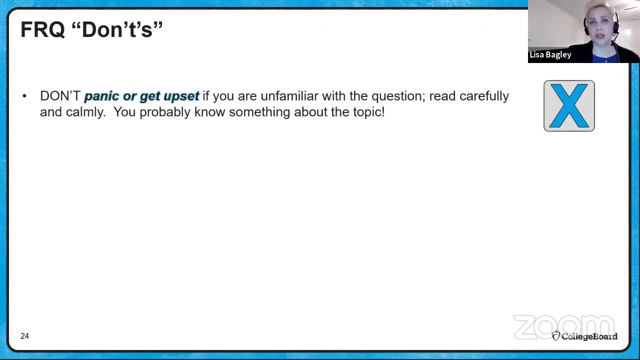 Get to the point of your response. For paper test takers, don't use pencil. Use a ballpoint or non-gel ink pen with blue or black ink. We'll still score you anyway, It's just harder to read. Finally, don't panic and don't get upset if you're unfamiliar with a question. 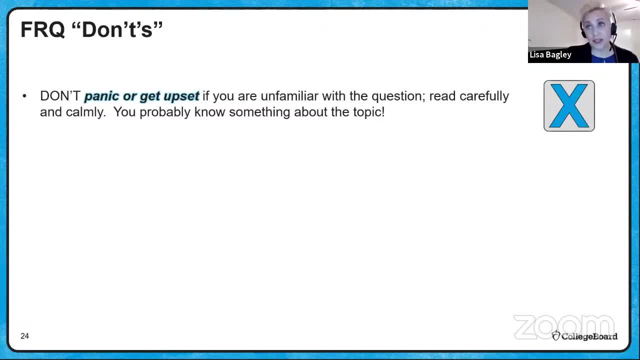 Take a deep breath, Read it carefully, Read it calmly. Think about the practice that you've had here, because you probably know something about this topic Somewhere in that brain of yours. For paper test takers, don't scratch out excessively One or two. 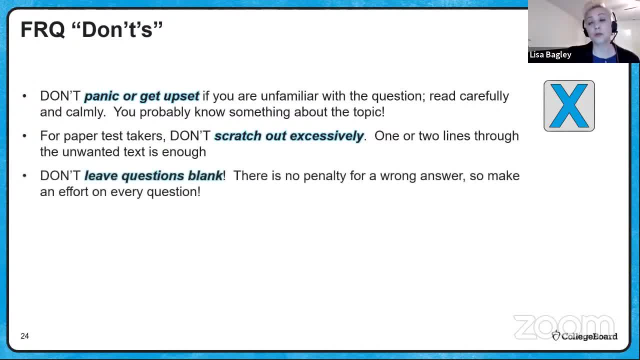 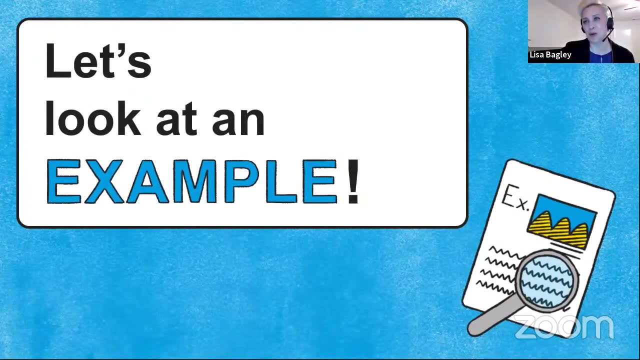 lines through the unwanted text is enough. Don't leave questions blank. There's no penalty for a wrong answer, So make every effort on every question And finally, don't quit. Don't quit. Give it your all. Let's look at an example. All right, here we go. Free response model question. 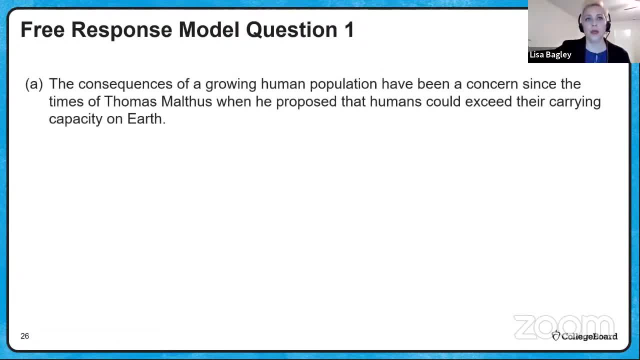 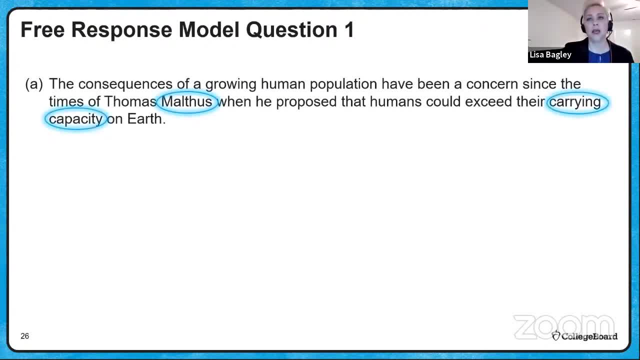 exceed their carrying capacity. on Earth There's Thomas Malthus, And so the concept we're talking about here is carrying capacity. Describe the concept of a carrying capacity for a species And describe how a change in the availability of a specific resource could affect the carrying. 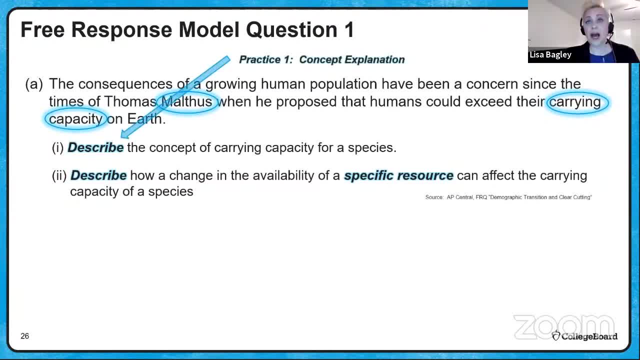 capacity of a species. This is concept explanation which is practice one. So the answer to that first part is: just give me what's the concept of a carrying capacity. The carrying capacity is the maximum population size of a given species that an environment can sustain without resource degradation. 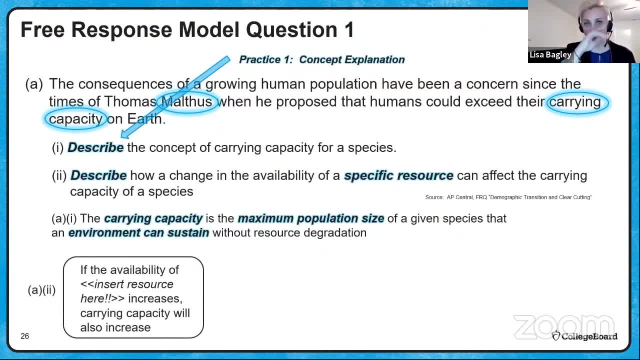 The second one has a little bit more to it. So notice that I highlighted a specific resource. They're wanting you to say a specific resource. They're wanting you to say a specific resource. They're wanting you to say a specific resource in your response And notice that I said: if the 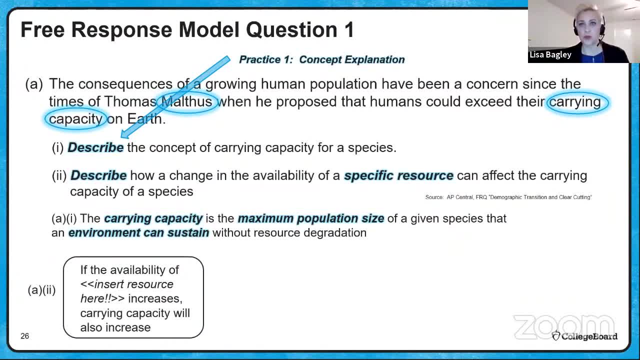 availability of insert resource here. So you could say something like if the availability of water, if the availability of food, if the availability of habitat. But you must name a specific resource because the prompt says specific resource. So let's see how we can model, answer this. If the availability of food, water, habitat increases, then the carrying capacity will also increase. Or if the availability of choose your resource decreases, the carrying capacity will also decrease. Or if the availability of your chosen resource changes, carrying capacity may not be. affected. But you have to link a specific resource and its availability going up or down to carrying capacity going up or down. So if the availability of food, water, habitat increases, then the carrying capacity may not be affected. But you have to link a specific resource and its availability going up or down to 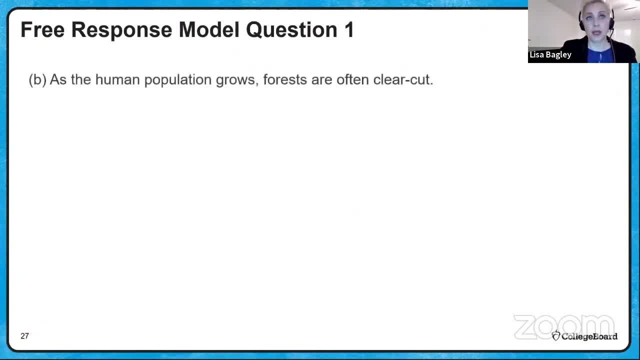 get that point right there. As the human population grows, forests are often clear-cut. Describe a negative effect of clear-cutting forested areas Concept explanation, By the way. so clear-cutting is topic 5.2.. So if you're not sure about the negative effect of 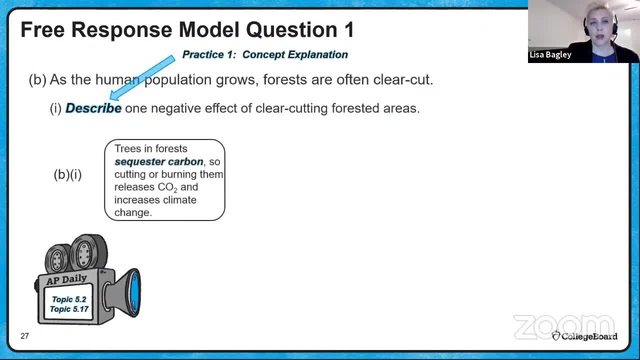 clear-cutting. check out video 5.2.. So trees sequester carbon. Burning or cutting them releases carbon, Which increases carbon dioxide, which increases climate change. Trees and forests absorb pollutants, So clear-cutting them reduces the absorption of. 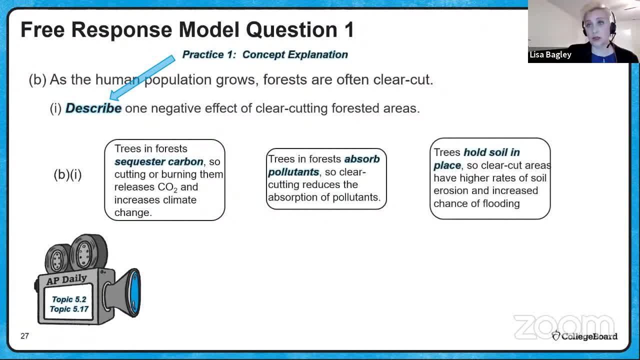 pollutants. Trees hold soil in place, So clear-cutting them. those clear-cut areas have higher rates of soil erosion and increased chances of flooding. Trees shade water and soil, So clear-cut areas have higher water and soil temperatures, which may lead to changes in. 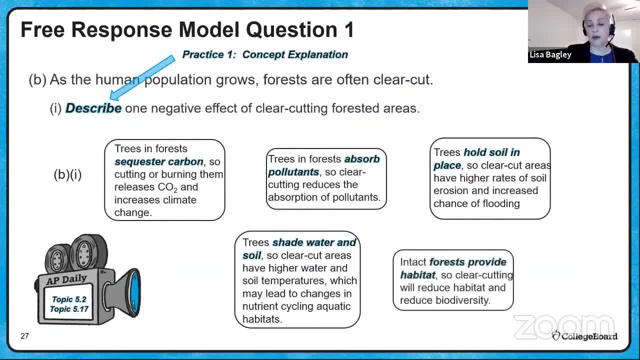 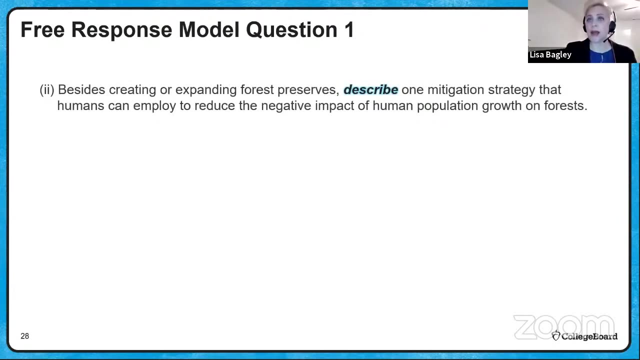 nutrient cycling in aquatic habitat. Finally, intact forests provide habitat, So clear-cutting them will reduce habitat and reduce biodiversity. Any of these are acceptable negative effects. They're all talked about in topic 5.2.. Besides, creating or expanding forest preserves, describe one mitigation strategy that humans can. 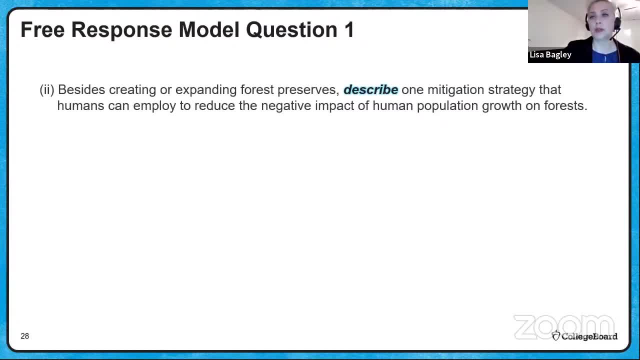 employ to reduce the negative impact of human population growth. So clear-cutting them will reduce habitat and reduce biodiversity. Any of these are acceptable negative effects. They're all talked about in topic 5.2.. Besides, creating or expanding forests describe one mitigation strategy that humans can employ to reduce habitat and reduce biodiversity. 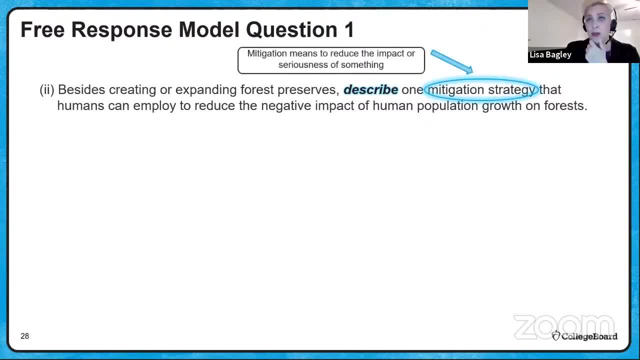 Hmm, what the heck is a mitigation strategy? Well, mitigation means to reduce the impact or the seriousness of something. So a mitigation strategy is something that would tend to reduce the impact, right, And of course it says, reduce the negative impact of human population growth. 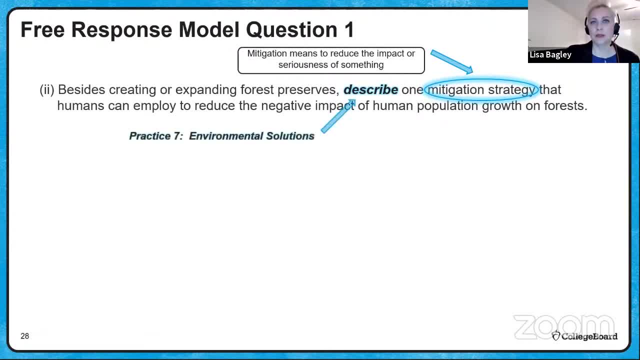 But the word mitigation can be a little bit freaky. That's environmental solutions. So you're going to provide me with some solutions. Those solutions would be in your sustainability, which is 5.17.. Practice sustainable forestry, where trees that are harvested can be replaced with seedlings that 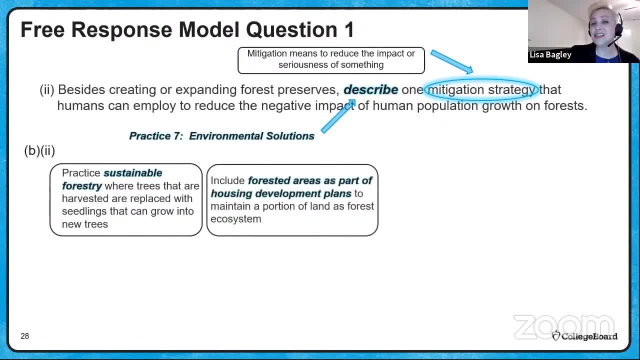 can grow into new trees. Include forested areas as part of housing development plans to maintain a portion of land as a forest ecosystem. Practice sustainable agriculture and food production. vertical farming- ocean farming to reduce the need to clear forested land for farming. Manage a forested area to extract some resources while still maintaining. 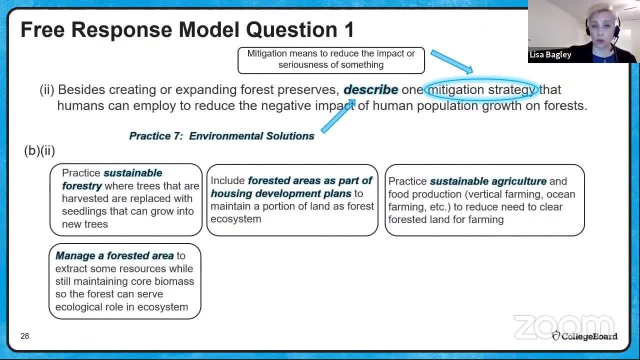 the core biomass, so the forest can serve an ecological role in the ecosystem, ecosystem services. Build up, not out, and construct or maintain high-density dwellings or neighborhoods that reduce the overall land use for housing developments. You don't have to cut down forest. 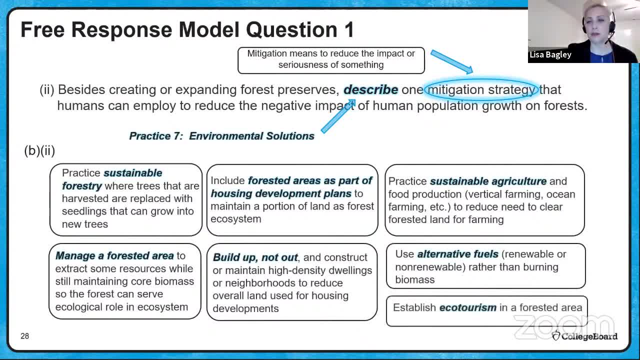 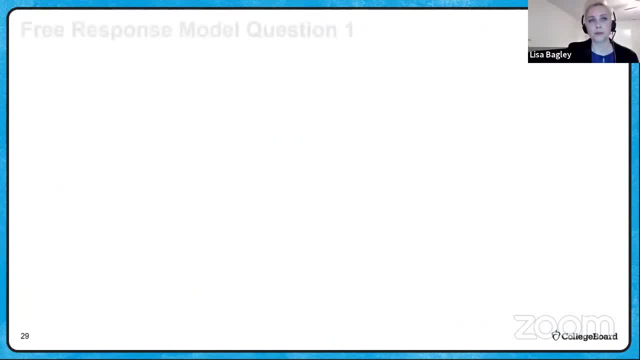 for that, Use alternative fuels rather than burning biomass And finally, establish ecotourism in a forested area. All right, lots of ways you could go there. And finally, still in part B, describe an additional benefit of the mitigation strategy. 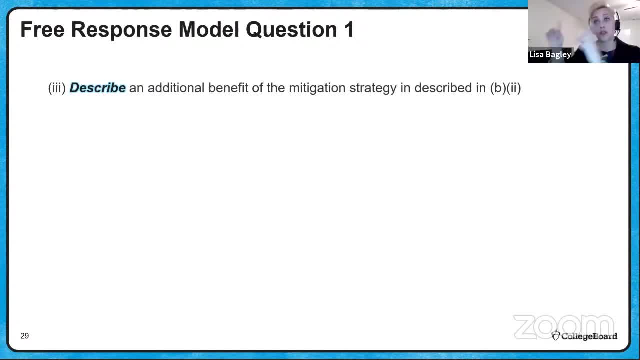 described in part BII. So your additional benefit has to match the mitigation strategy that you chose. So as we go through these answers, I'm going to say: if you chose this, then these are acceptable. If you chose this, these are acceptable. So here we go. Stick with me. 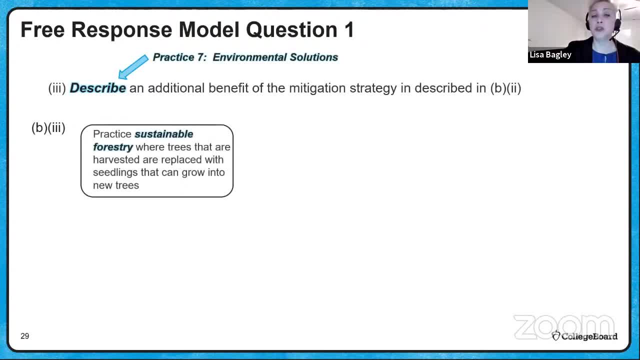 All right. So if you chose practicing sustainable forestry, an additional benefit of that is that sustainable forestry preserves biodiversity by maintaining a variety of plant and animal species, it protects soil and water resources, and it provides wood and resources for human use. If you chose, manage a forested area to do some extraction while still maintaining core biomass, 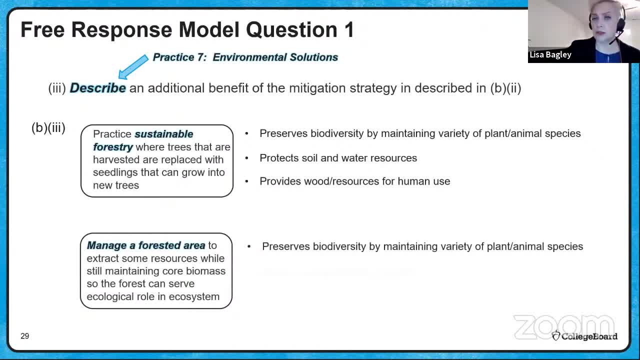 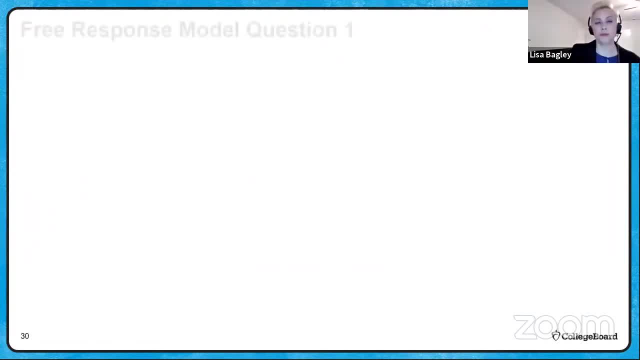 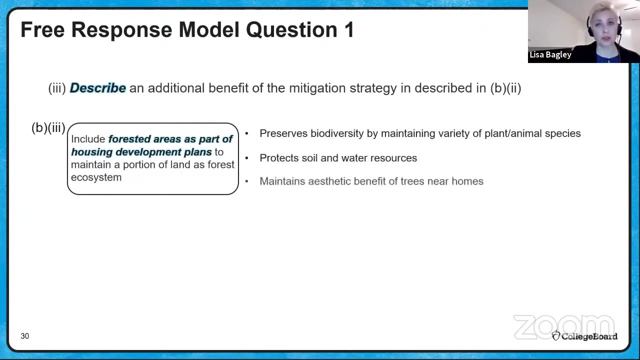 oh, look at that. It preserves biodiversity, It protects soil and water resources And it provides wood and resources for human use. We're still going on this one. All right, If you chose. include forested areas as part of housing development plans. it preserves biodiversity and it protects soil and water resources. 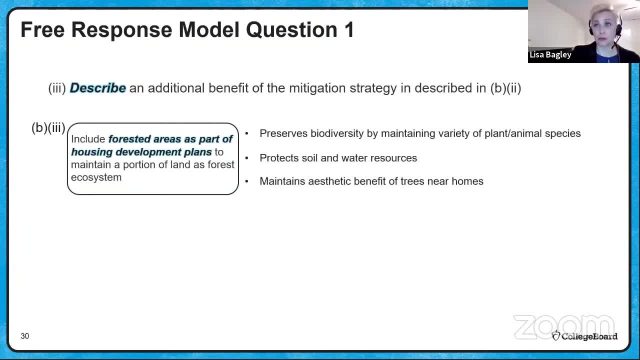 and it maintains the aesthetic benefit of trees near homes, which homeowners like. If you chose, build up, not out, and construct high density dwellings, then an additional benefit would be preserving biodiversity and protecting soil and water resources, as well as reducing the reliance on transportation fueled by fossil fuels. 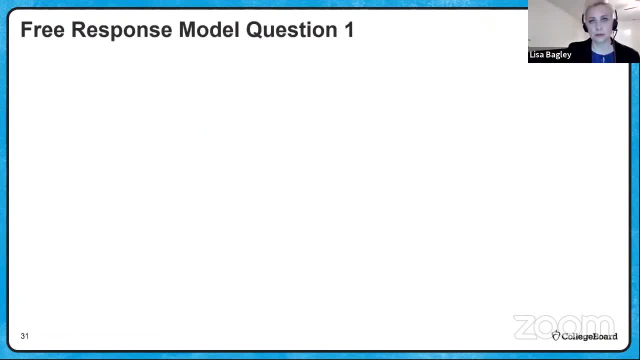 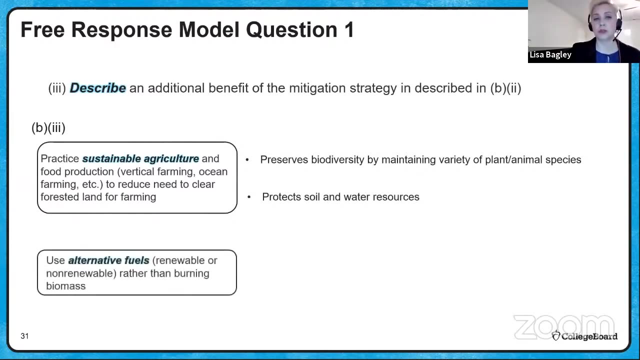 which decreases global climate change. overall, We're still going. If you chose to practice sustainable agriculture as your mitigation strategy, we will preserve biodiversity and protect soil and water resources. If you chose alternative fuels rather than burning biomass, it preserves biodiversity and protects soil and water resources. 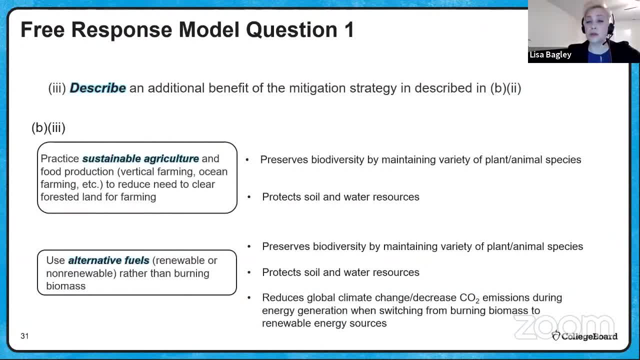 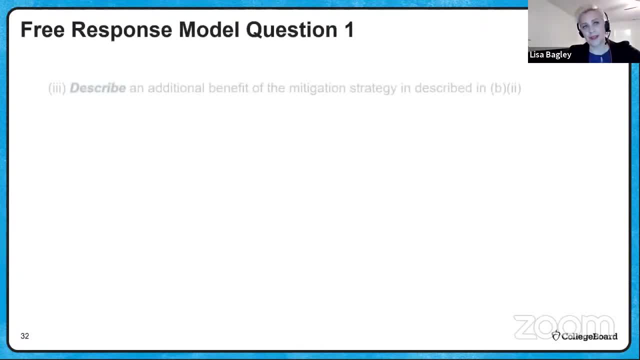 It also reduces global climate change and decreases CO2 emissions during energy generation, when switching from burning biomass to renewable energy resources. Finally, if you chose establishing ecotourism, it provides jobs and it brings money to the local economy. Those would be economic benefits. 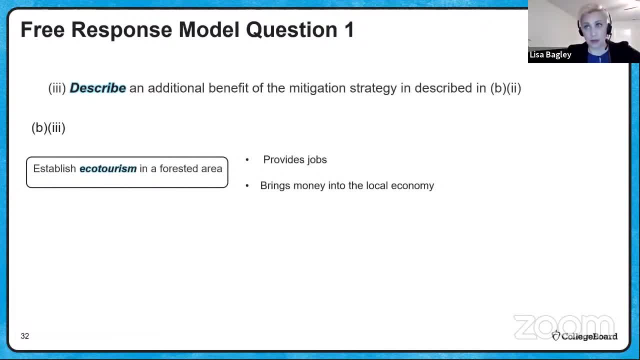 It doesn't specify in the prompt what kind of benefits it has to be. What did you notice about most of the model answers for the additional benefits of mitigation strategies, Preserving biodiversity and protecting soil and water resources? As a country industrializes, it often moves through demographic transition. 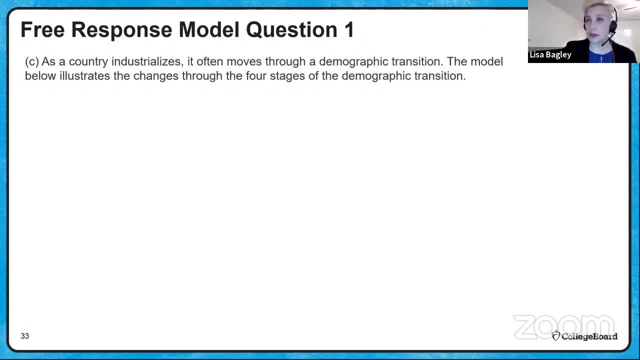 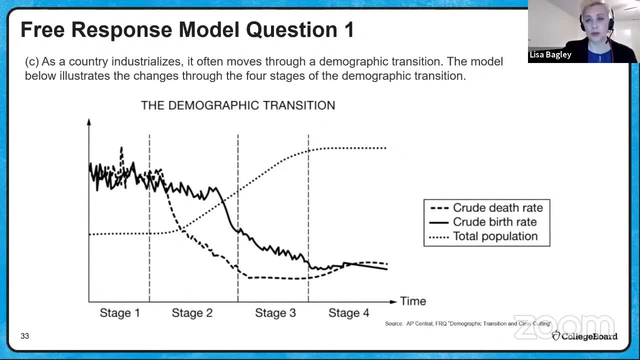 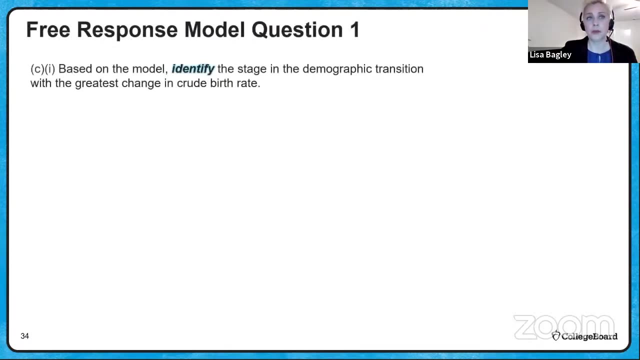 The model below illustrates the changes to the four stages of demographic transition. There is the visual of the demographic transition model that we verbally described in the previous slides. Notice there's a four stages and we've got a key there. Going to see that again. Based on the model, identify the stage in the demographic transition with the greatest change in crude birth rate. 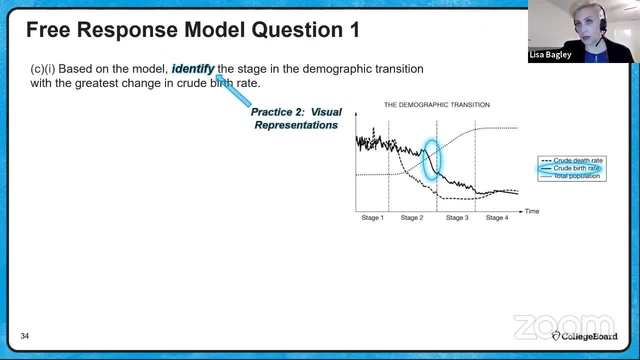 So this is a visual representation. Let's find the crude birth rate. There it is, And the stage with the greatest decrease or the greatest change- it could have been an increase, increase or decrease, but in this case it's a decrease- is stage two. 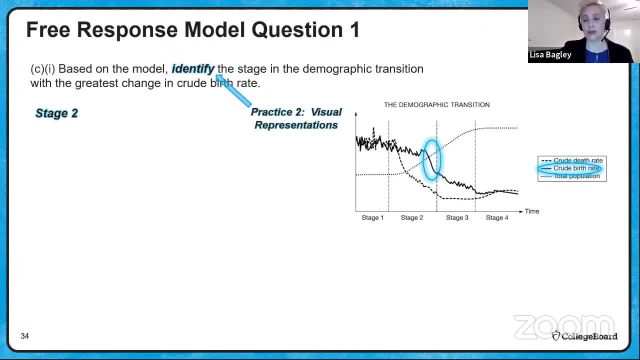 So if we were to take the slope of the line in that area, that one's got the greatest slope Based on the model. describe the relationship between the crude death rate and the crude birth rate that led to the trend in total population in stage two. 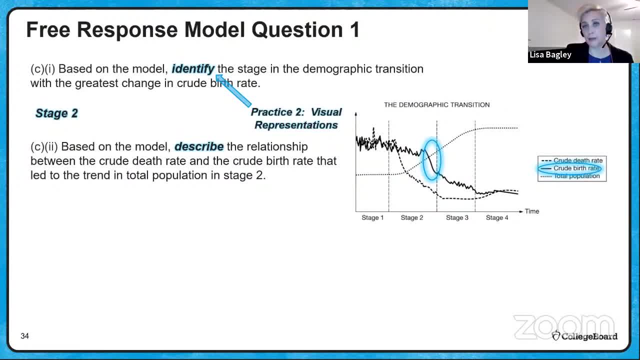 So, first off, we need to find total population, which is your dotted line. And when we look at that dotted line there in stage two, right, the total population is increasing, So the crude death rate decreased and the crude birth rate increased. 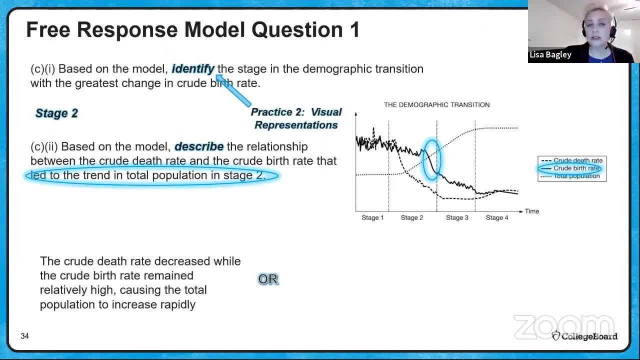 And well, it didn't really increase. It remained relatively high, which causes the total population to increase rapidly. That's what we're seeing there. That stage two is a rapid population increase, Or population growth rate can be increased. So that's what we're seeing there. That stage two is a rapid population increase. 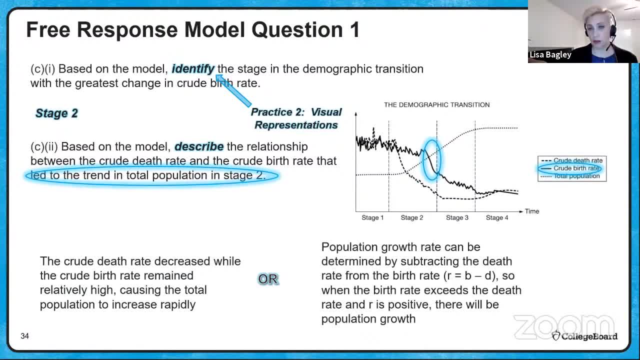 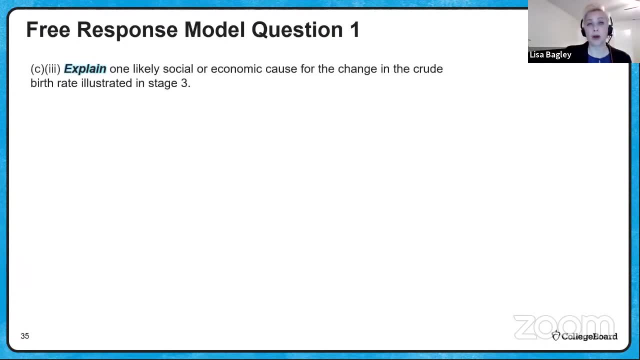 That stage two can be determined by subtracting the death rate from the birth rate. So when the birth rate exceeds the death rate, then the rate of growth is positive. So there'll be population growth. Could have gone either way. with that, Explain one likely social or economic cause for the change in the crude birth rate, as illustrated in stage three. 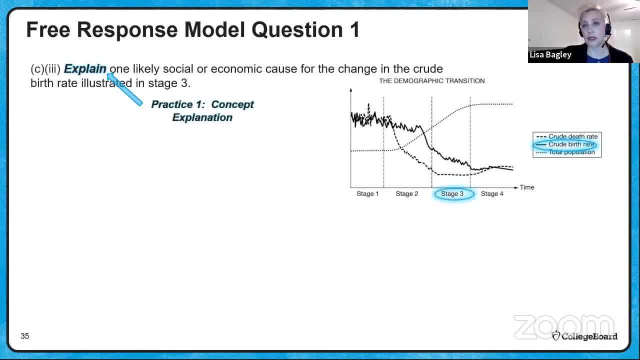 So let's first off find the crude birth rate in stage three, And there it is. So the question is: what's the trend that you observe there? Because there's a change, and that's what the question is asking you to explain. 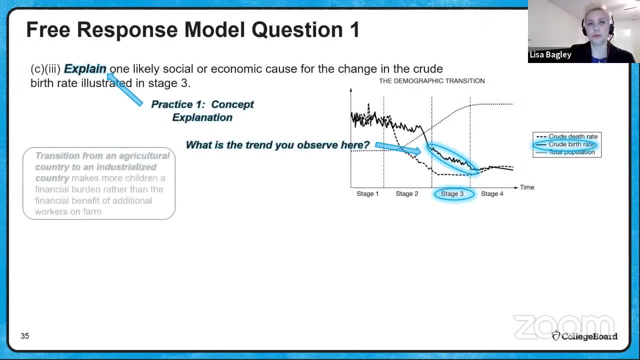 So there is a decrease in your crude birth rate. This could be caused from a transition from an agricultural country to an industrialized country, And that change makes more children a financial burden rather than a financial benefit. A rise in relative affluence of the country can affect the status of women. 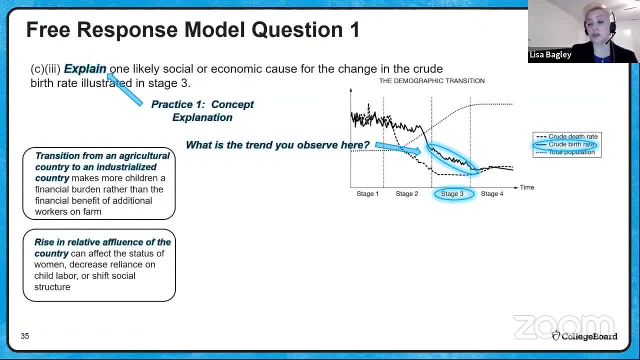 There's a decrease in the birth rate, It's a decrease in reliance on child labor or a shift in the social structure. Expansion of women's status and access to education, to economic opportunity or political power increases the age at which a woman first has her babies. 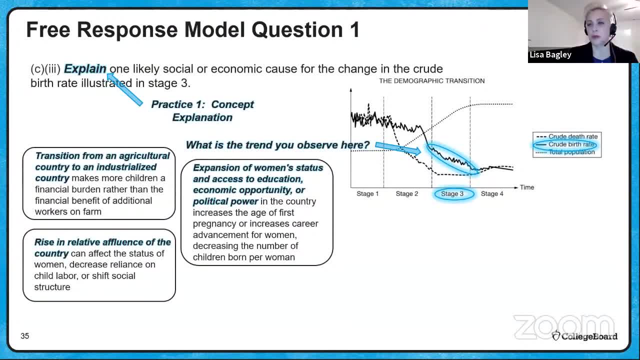 and increases career advancement for women, which would lead to a reduction in birth rates. Increased access to contraception, which enables family planning and decreases fertility rates. The increased average age at marriage: If you marry later, you tend to have fewer babies, which reduces the overall number of children per woman. 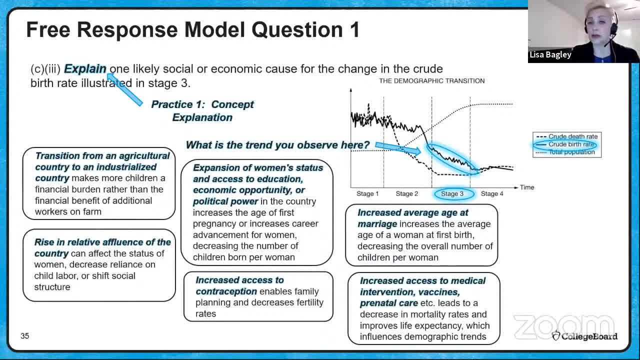 Increased access to medical intervention, vaccines and prenatal care leads to a decrease in mortality rates and an increase in life expectancy. Any of those would account for that decrease in crude birth rate shown in stage three. We're finally at part D During a demographic transition. 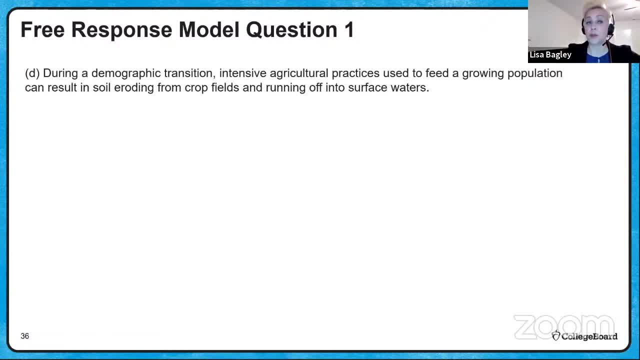 intensive agricultural practices used to feed a growing population can result in soil eroding from crop fields and running off into surface waters. Make a claim. there's your. practice seven that proposes an effective long-term solution to minimize the erosion of topsoil into surface waters. 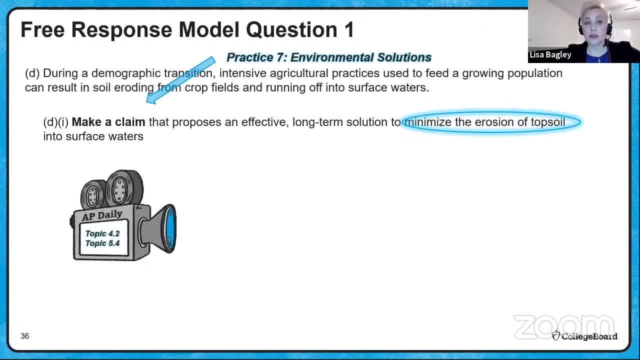 So we're going to provide a solution. Here we go Again. soil is topic 4.2.. And 5.4 is agriculture. So you can maintain and plant vegetated buffers between surface waters and crop fields. You could create retention ponds to capture the eroded soil. 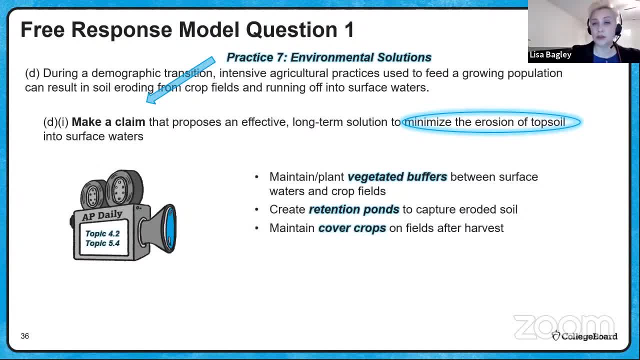 You could maintain cover crops on fields after harvest to minimize erosion. You could use no-till agriculture, strip cropping, contour plowing or terracing. Any of those would be acceptable long-term solutions to minimize the erosion of topsoil. Next slide. 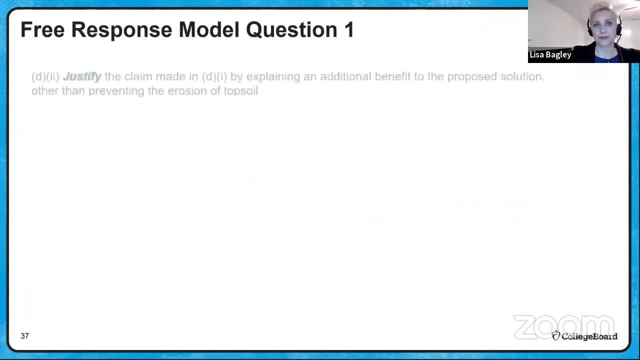 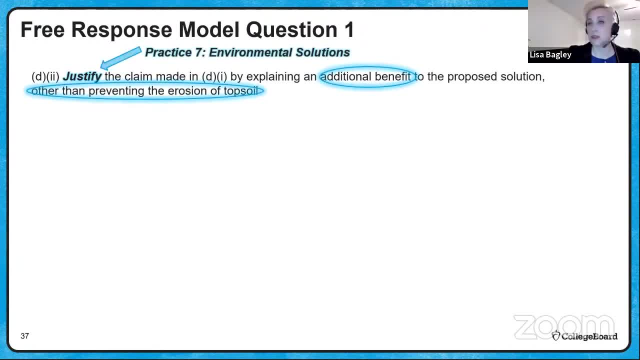 Additional benefit Justify it. This is again practice seven. All right, So an additional benefit, other than preventing the erosion of topsoil, If you chose planting vegetated buffers, it creates habitat to maintain biodiversity, creates habitat for crop pest predators, which provides a natural method of 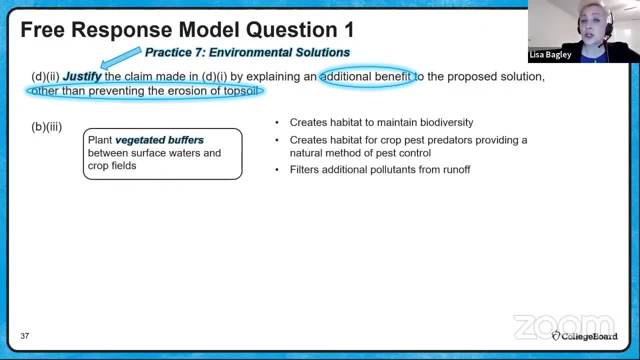 pest control, and these vegetated buffers filter additional pollutants from runoff. It also recharges groundwater by slowing the flow of runoff, which allows for infiltration. If you chose creating retention ponds, this would create a habitat for aquatic species, which helps maintain biodiversity. filters additional pollutants from runoff. 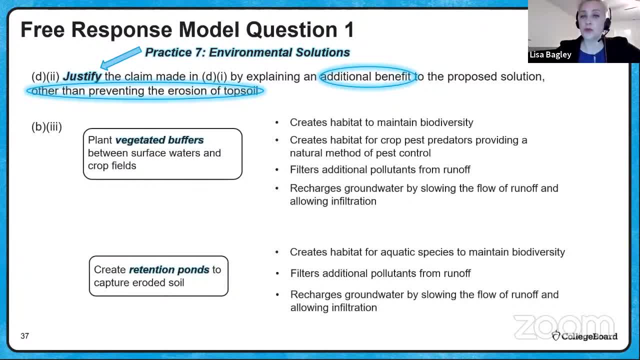 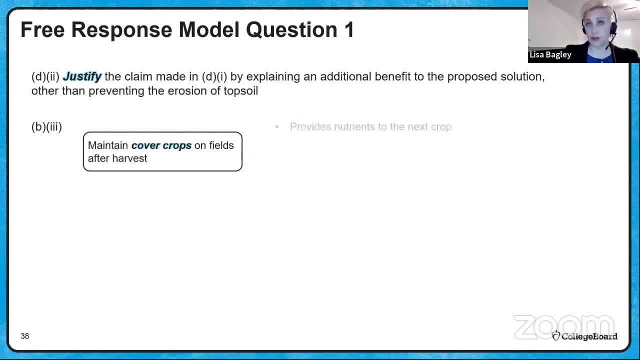 and recharges groundwater by slowing the flow of runoff and allowing for infiltration. If you chose, maintaining cover crops on your field, that provides nutrients for your next crop. So we're talking a lot about agriculture here. It suppresses weeds and it filters additional. 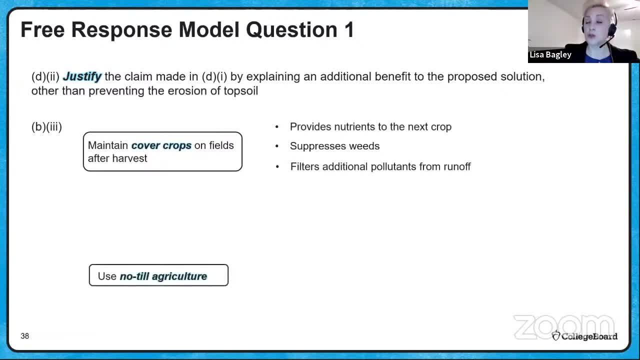 pollutants from runoff. If you chose using no-till agriculture, that reduces fuel requirements needed on your farm. It also reduces the release of greenhouse gases associated with mechanized agriculture, which decreases global climate change. If you chose using strip cropping, contour plowing or terracing, these improve crop yields. they maintain soil fertility. 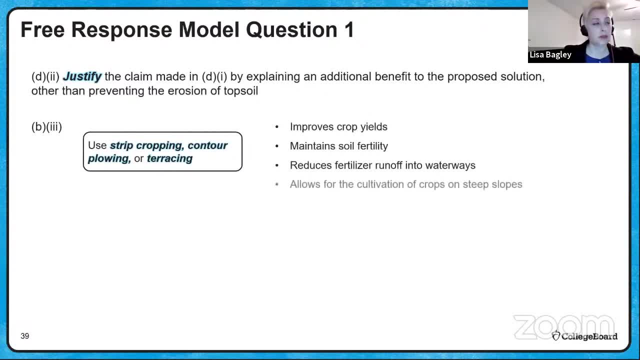 and they reduce fertilizer runoff into waterways. Oh, and it also allows for the cultivation of crops on steep slopes. So all of this is practice seven. Practice seven is heavily tested on the FRQ portion of the exam. Both questions two and three will ask you to provide environmental solutions and to justify. 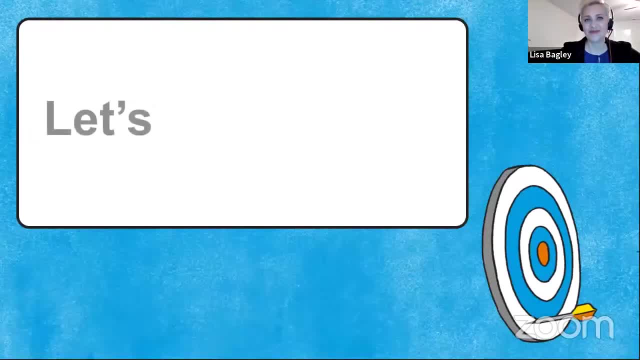 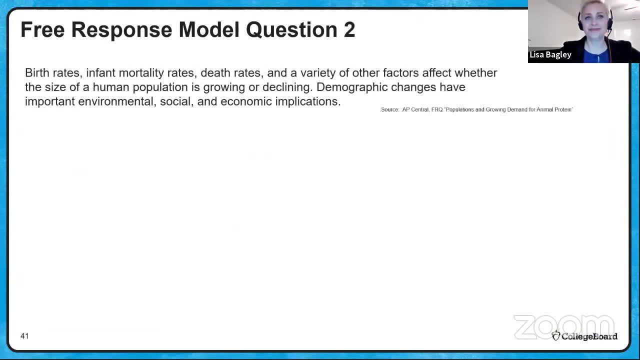 them. You'll see this again in model question two. All right, deep breath. These are long. All right, here we go. Birth rates, infant mortality rates, death rates and a variety of other factors affect whether the size of a human population is growing or declining. Demographic changes: 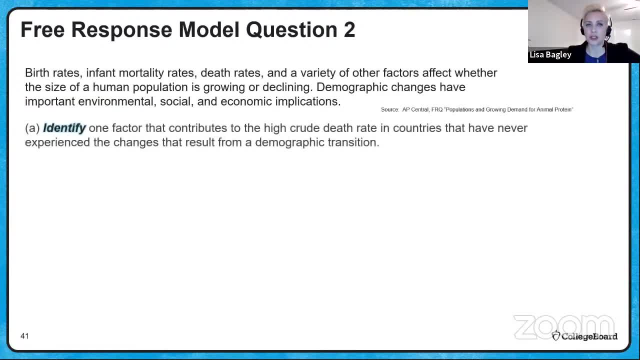 have important environmental, social and economic implications. Identify one factor that contributes to the high crude death rate in countries that have never experienced the changes that result from a demographic transition. Okay, this is practice one, And a lot of this actually links in with the previous one. 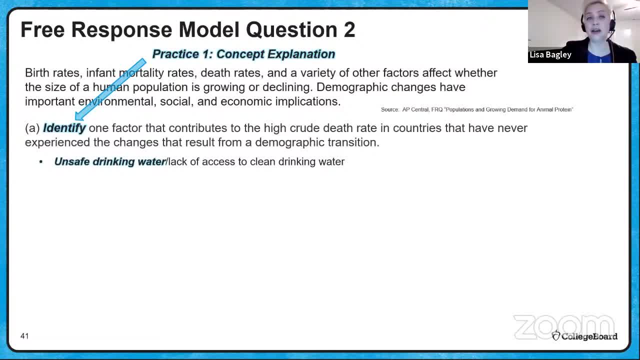 Okay, this is a little more about the ranks And I'll show you a little bit of the key differences and individual categories. So the first one is with the data entry: how do you make a decision? So, again, we're going to say that the data that's being generated 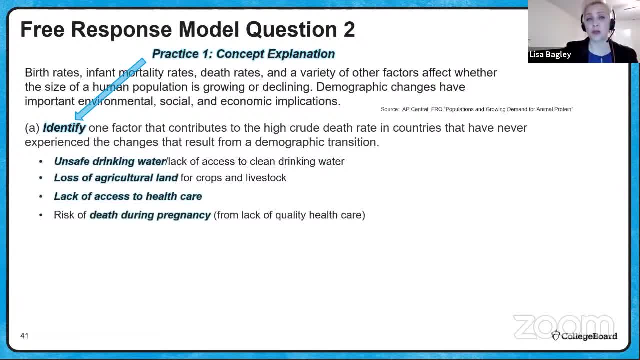 is not only a result of a specific, specific group of factors that are relevant to a particular population subsection. A low tapi or a high people who are associated with those groups are not the target people at all. So you know, if you look at, for example, the articles, 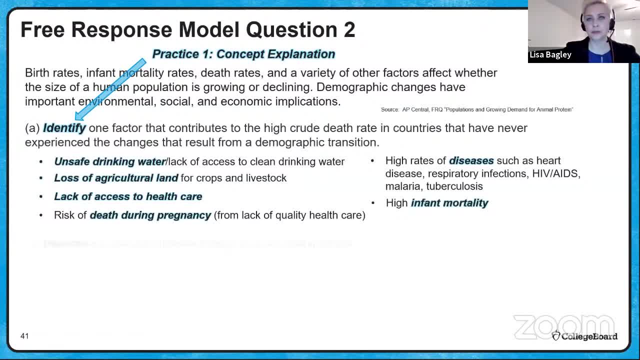 that would show the status of a particular population subsection in the data entry. that's a、. you know, the higher the number of percent of people that are associated with that. you know it's. you know, the higher the number of percent, the higher the number of percent. 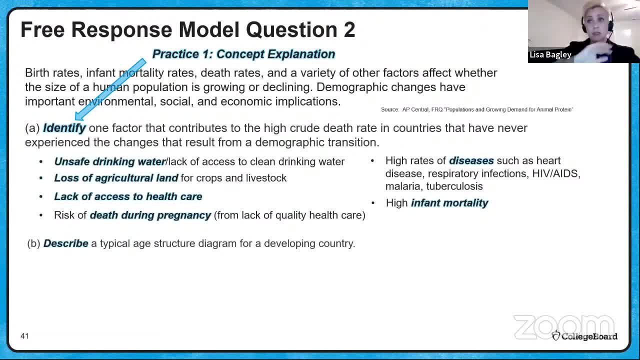 And that's an identified prompt. So you just need to tell me what it is and move on. Describe a typical age structure diagram for a developing country. A developing country has a pyramid-shaped age structure diagram. There's more individuals in the younger cohorts and there's a broad base to that pyramid. 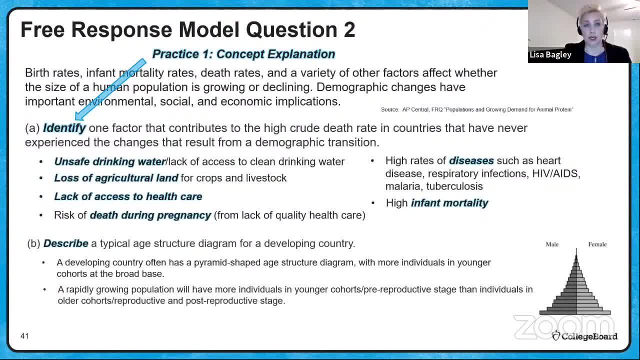 They look kind of like the one that I just popped up on the screen. A rapidly growing population will have more individuals in the younger cohorts and the pre-reproductive stages and less in the older cohorts. Any of these points, any of these, would be acceptable answers. 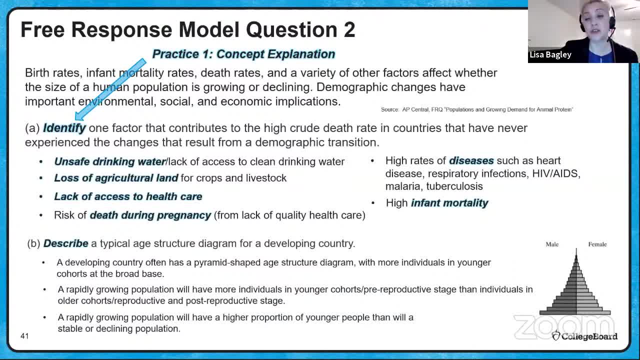 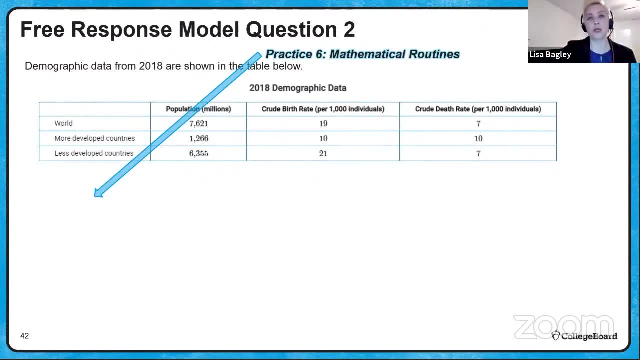 Or a rapidly growing population will have a higher proportion of younger people than will a stable or declining population. But you need to describe it for me, All right. So demographic data from 2018 are shown in the table below, So use the data in the table to answer the following questions. 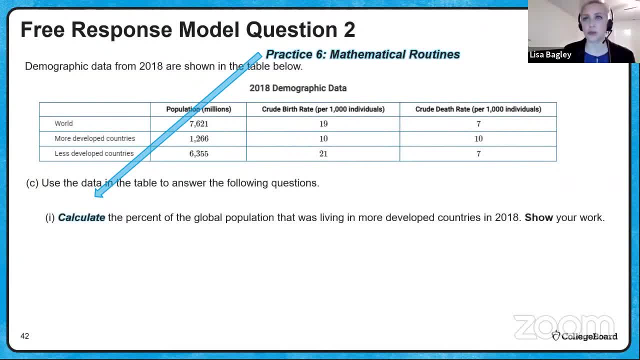 My animation was a little off there. This is obviously practice six, which is mathematical routines. So we've got world, more developed countries, less developed countries. We have population in millions, crude birth rate per 1,000, crude death rate per 1,000.. 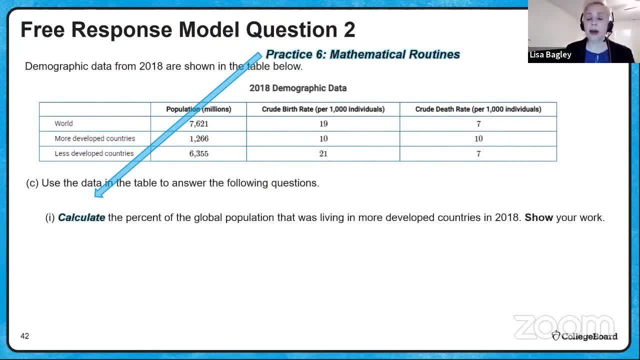 So, again, I like to take a visual of what I'm looking at. So we're going to calculate the percent of the global population That was living in more developed countries in 2018, OK, So the way to do this, this is our formula. 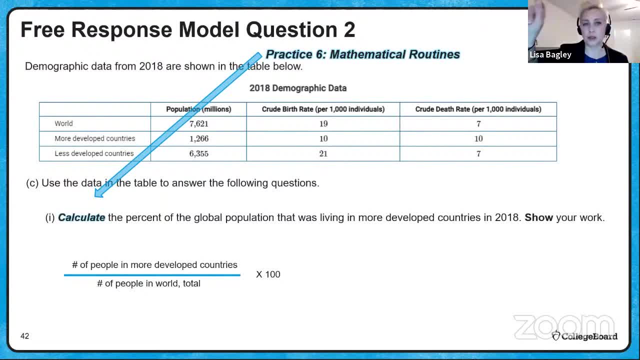 So it's the number of people in the more developed countries, And our denominator, our divisor, is the number of people total in the world, And then times 100. So first find your more developed countries number. There she blows, Then your world number. 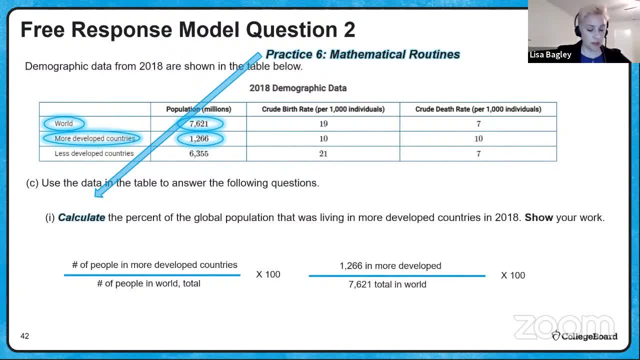 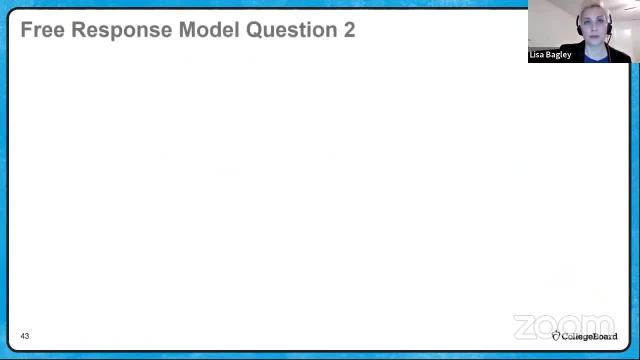 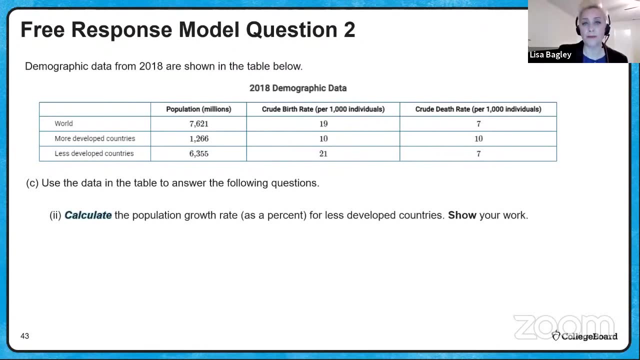 There it is. So when we plug those numbers in to our formula, this is what we got: Approximately 16.6%. OK, We're going to use the data to answer the following questions. We're going to calculate the population growth rate as a percent for less developed countries. 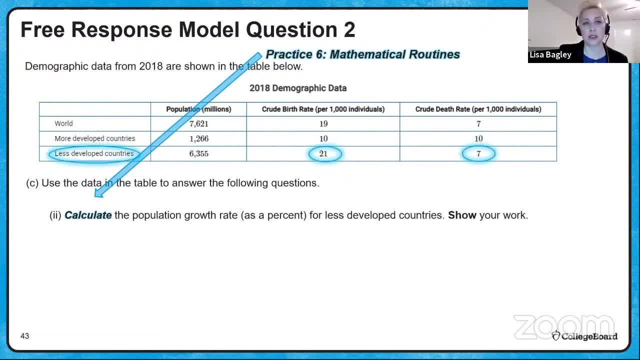 And we're going to show our work. Again, this is mathematical routines. There's our less developed countries And we want our crude birth rate. So we have 21 births Per cent Per thousand people, Minus seven deaths per thousand people. 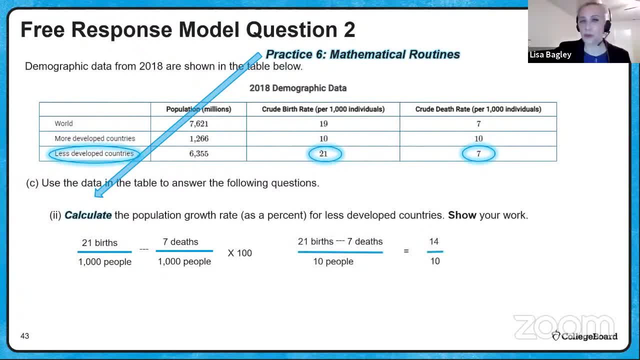 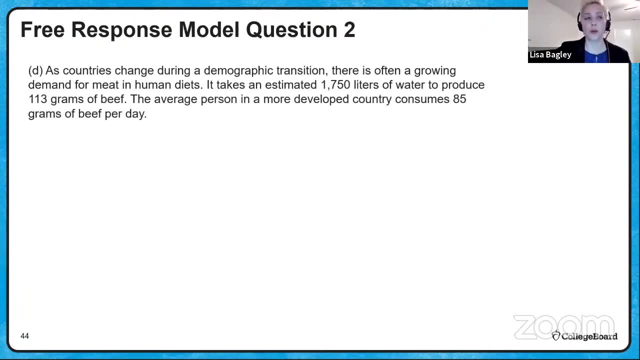 Times 100. And when we actually we're going to reduce that. So we've got 21 births minus seven deaths Divided by 10. Equals 14 over 10. Which equals 1.4%. As countries change during demographic transition, there's often a growing demand for meat in human diets. 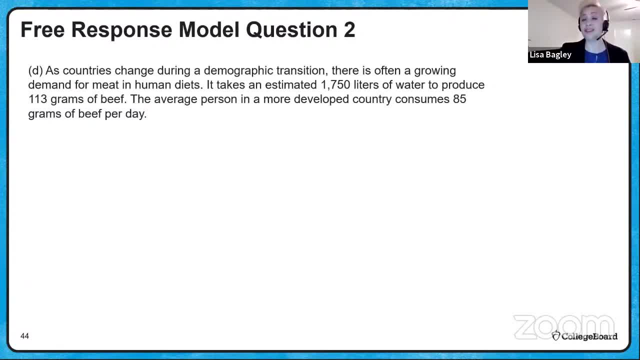 It takes an estimated 1,750 liters of water to produce about 100. The average person in a more developed country consumes about 85 grams of beef per day. So we've got some important numbers in there. Calculate the amount of water needed in liters per year to produce the beef consumed by one person in a more developed country. 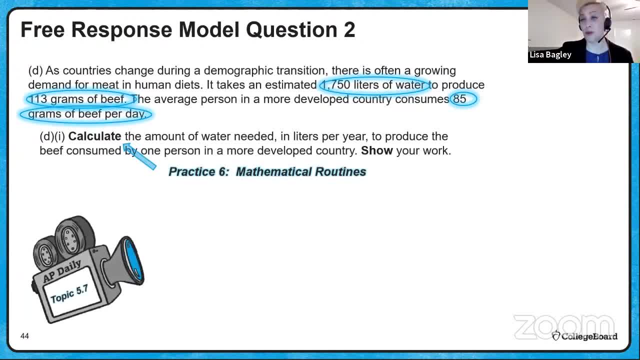 And, of course, show your work. Here we go. This is topic 5.7,, by the way, 85 grams per one day Times 365 days in a year, Times The liters of water per grams of beef yields 4.8 times 10 to the 5th liters of water per year. 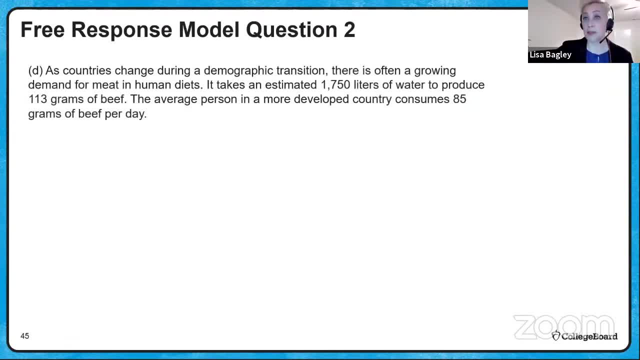 Dimensional analysis. Same prompt, Different question. Make a claim to propose a solution that would reduce the amount of water required to produce enough food for individuals. Make a claim We're going to reduce the amount of water. Environmental solution: Here we go. There's a lot of them. Eat less meat. Produce plant-based protein sources. Use drip irrigation for crops. Plant local or native crops that do not require as much water. Plant GMO crops that do not require as much water. Switch from water-intensive livestock farming like beef to less water-intensive livestock farming like chicken. 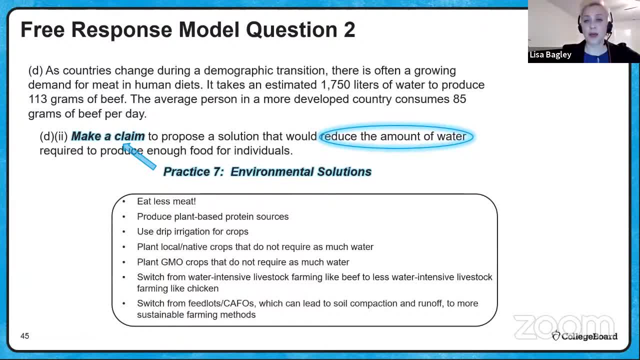 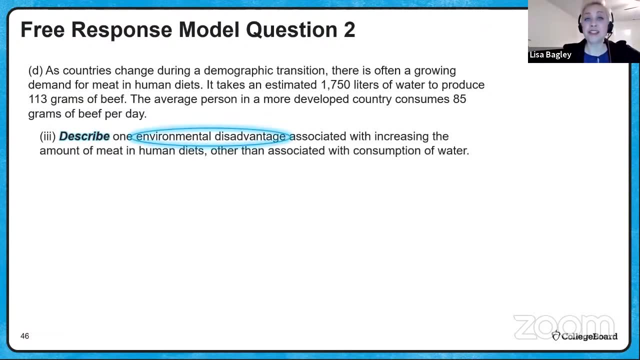 Switch from feedlots or cathos, which can lead to soil compactation and runoff, to more sustainable Farming methods. Any of those would reduce the amount of water required to produce enough food for individuals. Same prompt, Different question Describe one environmental disadvantage associated with increasing amount of meat in human diets. 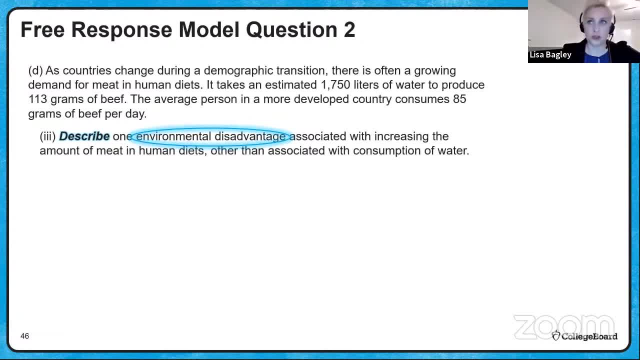 other than the associated with the consumption of water, which we just talked about Again. environmental solutions: More land is required to produce the same number of calories from meat as from plants. The use of animal feedlots to raise animals generates large amounts of waste. 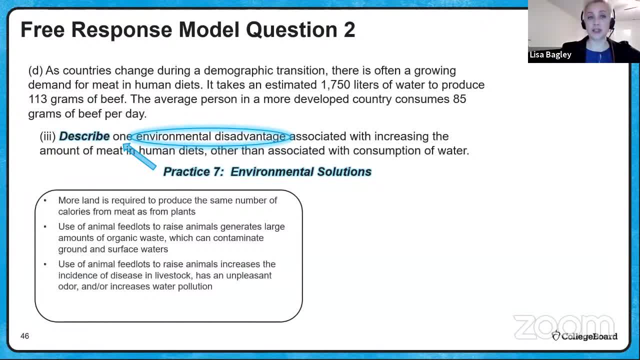 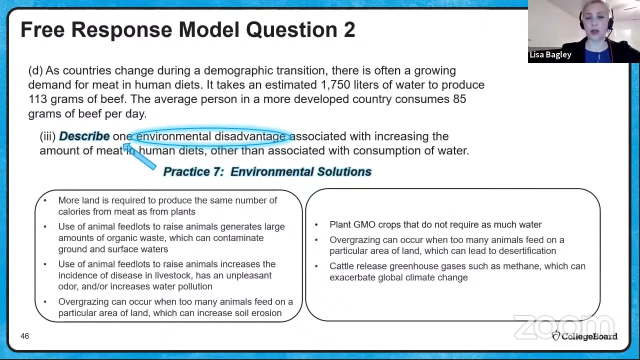 This contaminates ground and surface waters, Animal feedlots, increases incidence of disease in livestock, has an unpleasant odor and increases water pollution. Overgrazing can occur because we have too many animals in one area And cattle release greenhouse gases such as methane, which can exacerbate global climate change. 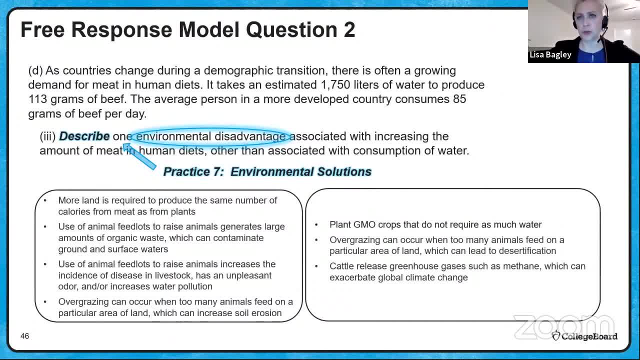 Sorry about that, guys. I had a leftover from the previous one, So we've got our overgrazing, which is on both those slides there, and then cattle releasing greenhouse gases such as methane. So there's one, two, three, four, five of them, including that methane. 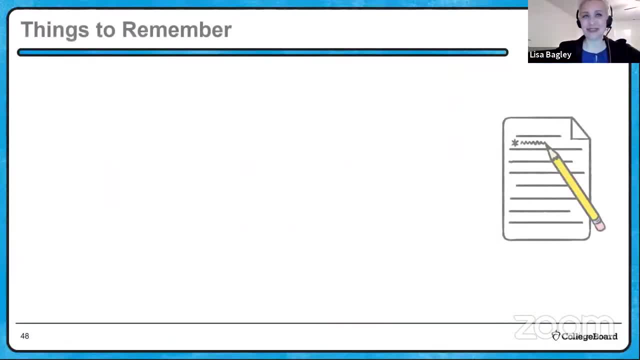 Whoops All right. So what should we take away from today? Things to remember. Remembering a few key do's and don'ts for your free response questions can increase your scoring potential. In order to earn full credit, you must show all your math work as well as the units. 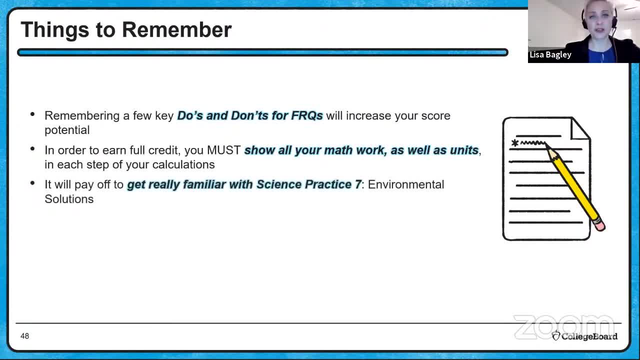 In each step of your calculations. it's going to be really, really good to get familiar with science practice seven, which is environmental solutions, and how to justify your answers there. Be sure to reference a stimulus image, graph or table if you're asked to provide evidence and you have a graphical stimulus. 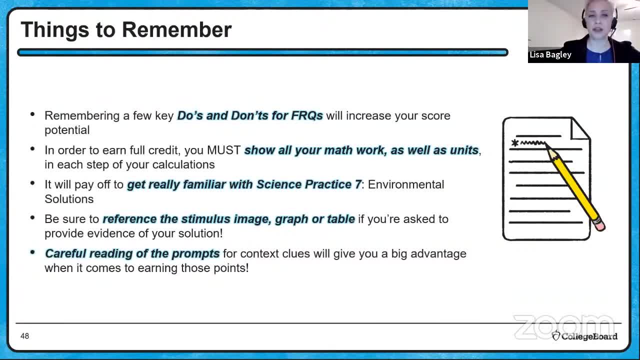 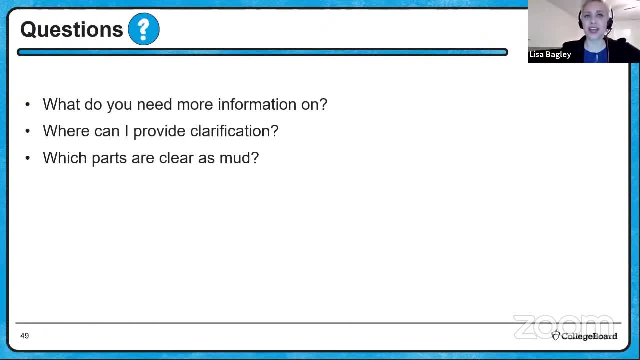 And, of course, careful reading of the prompts for context clues will give you a big advantage when it comes to earning points. So, once again, I am soliciting your help with clarification and information. What can I do? What can I do to make things clearer and better? 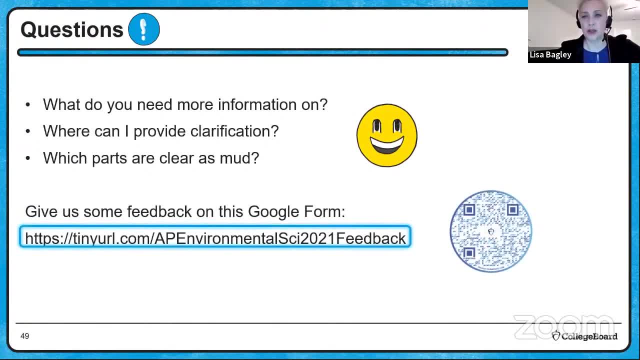 There's your Google feedback form. There's your QR code. Lay it on me. I'm going to give you a second to grab that. Of course, I'm going to answer some submitted questions. You might get a shout out at the beginning of AP Daily Live video three. 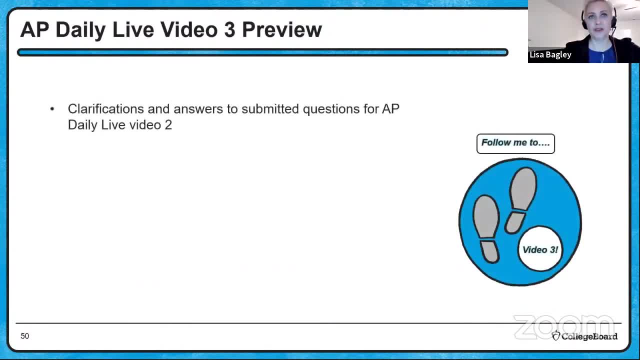 Be sure to tune in to us Preview of that video. We'll go with clarifications and answers to submitted questions for AP Daily Live video two, Just like we did today, Content review on Earth systems. Lots of visual models in this one. 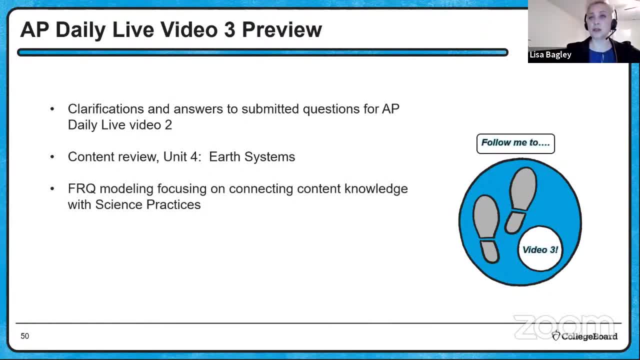 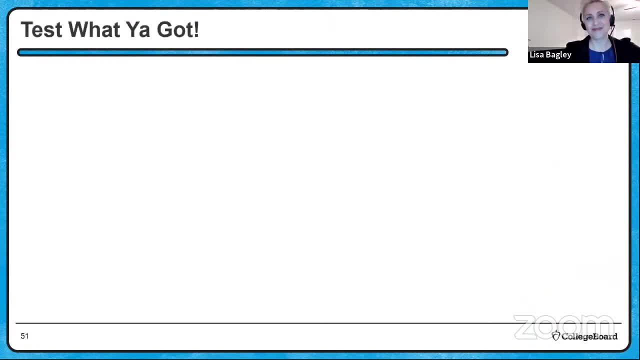 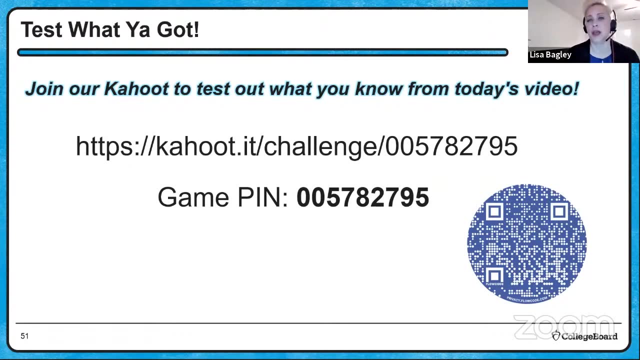 Of course, FRQ modeling with connecting science practices to content, knowledge, Interactive practice on concepts in video three. Here's your Kahoot Test. what you got, There's your Kahoot URL, your game pin and your QR code. Game pin is 0057827. 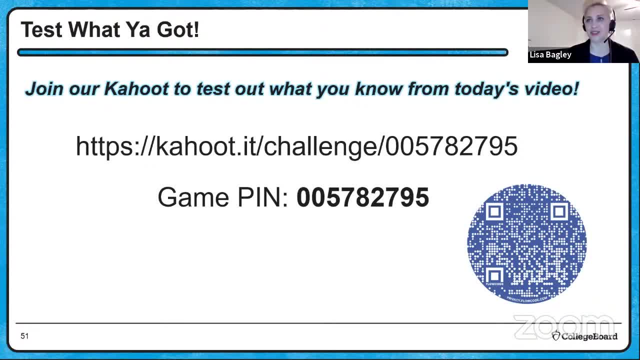 I love to see an everybody play yesterday. Have at it, friends, As always. thanks for watching and I'll see you tomorrow night.